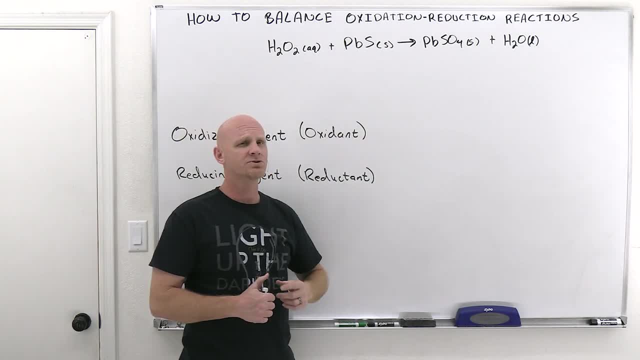 the first one is this reaction: right here We're going to balance it, And the thing that makes this so tricky is you got to balance out the electrons. it turns out Again with a redox reaction. electrons are being lost by one's BC. 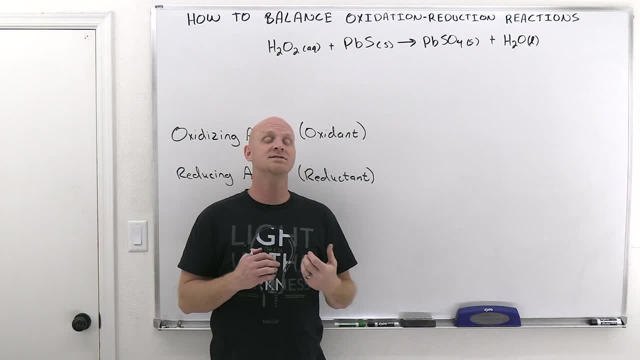 That's the species being oxidized and gained by another species. That's the species being reduced. It's an electron transfer reaction And you've got to keep track of those electrons, because the electrons that are lost are the same electrons that are gained and it has to balance out to be 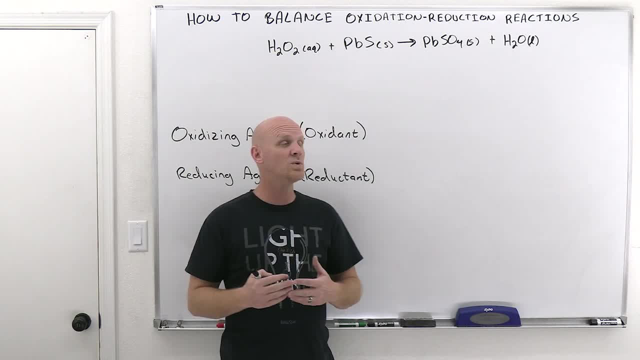 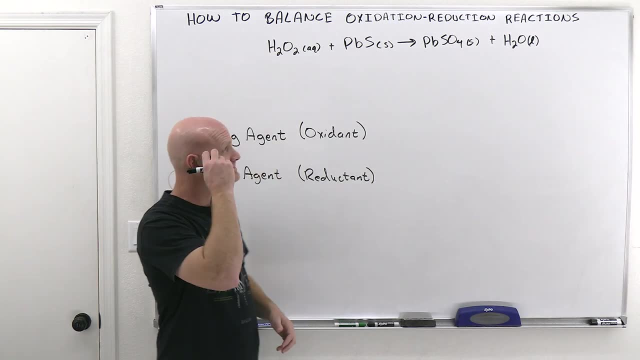 the same number of electrons, And so, in addition to balancing all the elements which you can see, you have to balance out the electrons which you can't, And that gets to be a little bit tricky, as we'll see. All right, before we get there, though, I just want to take a look at this a. 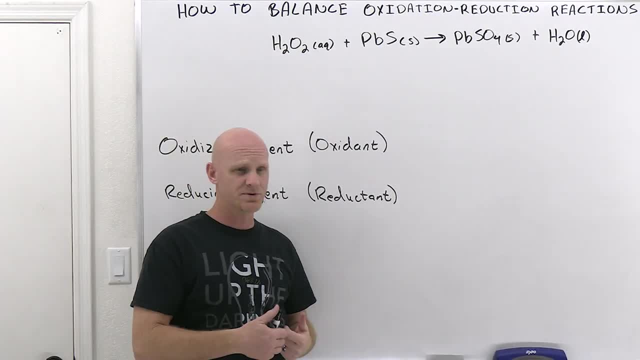 little more depth in the context of redox reactions. So we're going to go ahead and see who's being oxidized, who's being reduced and stuff, and we'll assign oxidation states to figure that out. And so in hydrogen peroxide it's one of the examples we did in the last lesson. 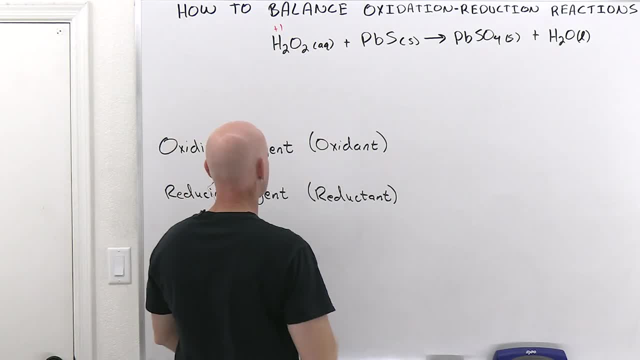 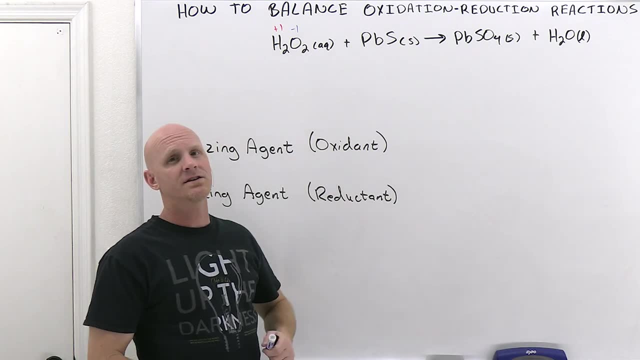 You'd assign hydrogen first as plus one and that's going to leave oxygen to be minus one to balance. So in the next one here we've got lead, and lead is below the staircase. It's not a transition metal technically, but it is below the staircase. We kind of treat it the same and 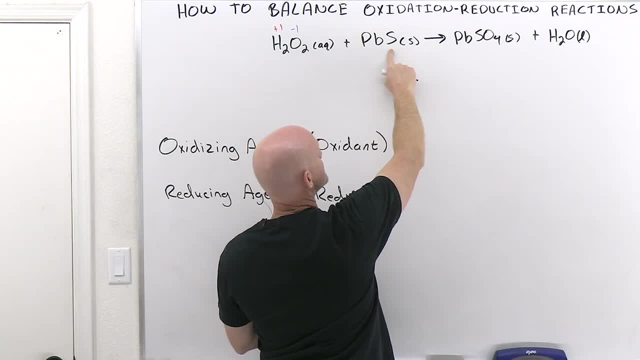 we'll balance them first, And he's going to have to be being with a sulfide monatomic ion here, which is minus two. That means lead's going to have to be plus two and that means sulfide as a monatomic ion is. 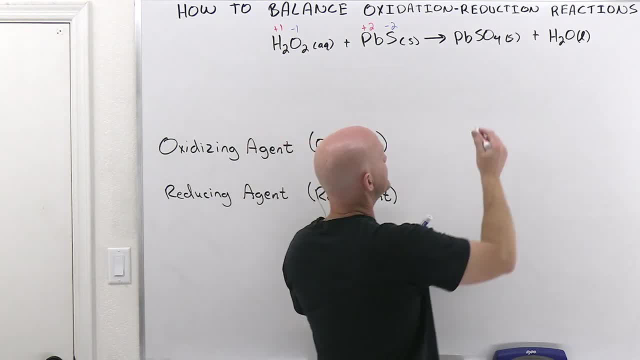 definitely going to be minus two. On the other side of the reaction, lead here with sulfate is still plus two, since sulfate as a polyatomic ion is minus two. So after that we'd assign oxygen with his normal oxidation state, since he's more electronegative- as minus two. And 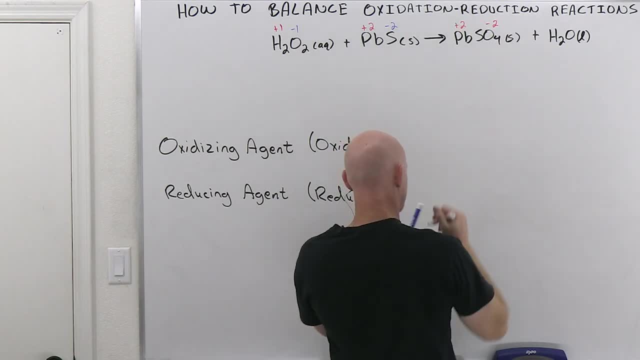 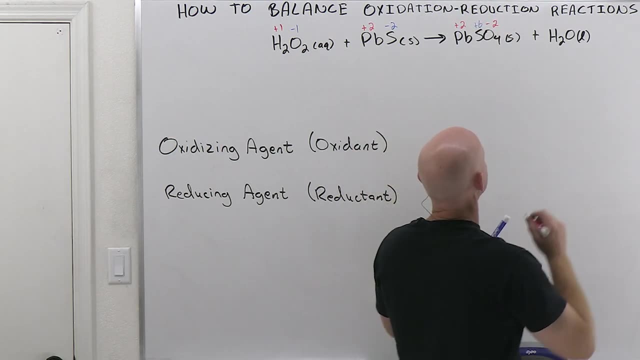 there's four of those, for a total of minus eight. With the plus two lead, we need another plus six on the sulfur to make this balance out to zero for a neutral compound. And then finally, in water, we'd assign hydrogen first as plus one and then oxygen second, therefore as minus two, to balance. 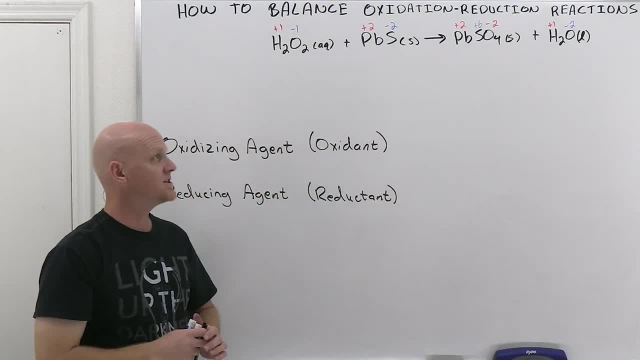 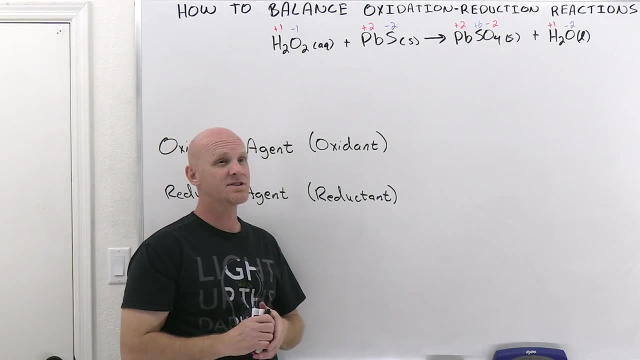 out to zero. And now we've assigned all our oxidation states. And again, you might not be as quick to assign them as this, but, word of the wise, get quick at assigning oxidation states. It will save you a ton of time in different places on this exam. All right, So we want to look at 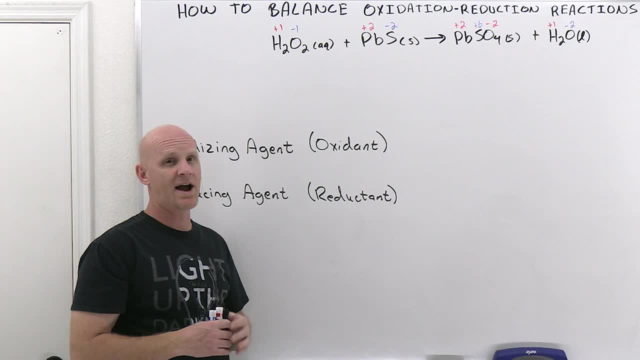 who's changing oxidation states, because that's kind of the hallmark of an oxidation reduction reaction, or redox reaction for short: Find those who are gaining or losing electrons, and we find those by seeing who's changing oxidation states. So, if we look here, hydrogen- here is plus one. Well, 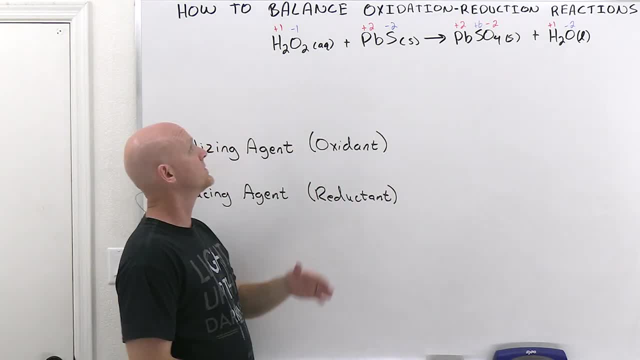 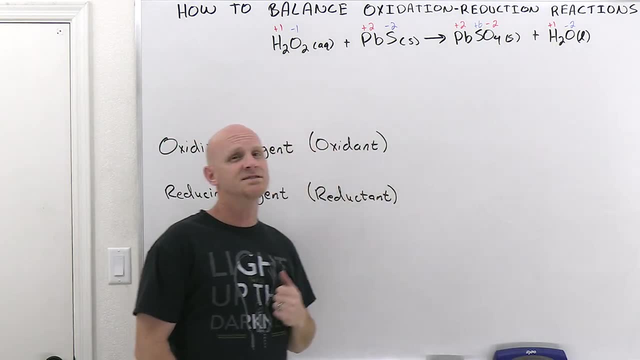 hydrogen over here is still plus one. There's no change there. But look at oxygen. Oxygen's going from minus one here to minus two in these two places. Oxygen is indeed changing And going from minus one to minus two. no matter how you slice it, his oxidation state is getting more negative. 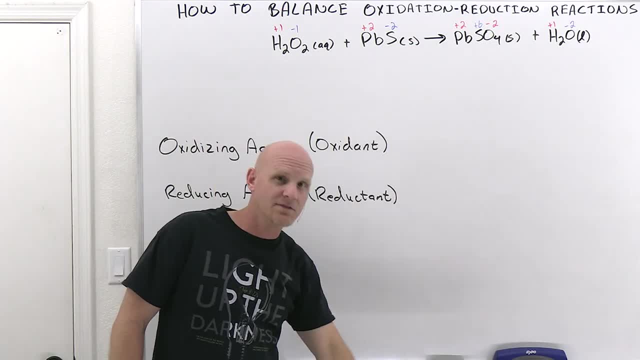 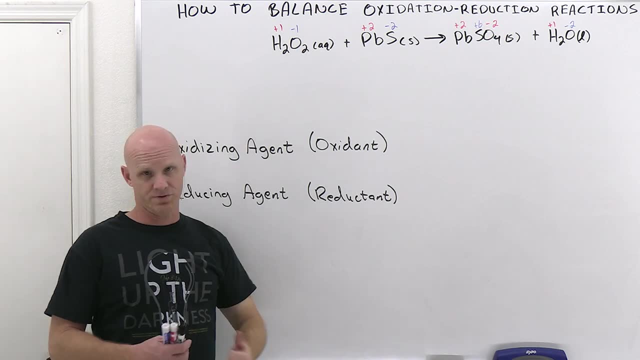 Well, that's going down. Whether it means less positive or more negative, that means going down, And that's why they call it being reduced, And so oxygen is the element that is being reduced. Okay, You could also say, instead of just saying oxygen. 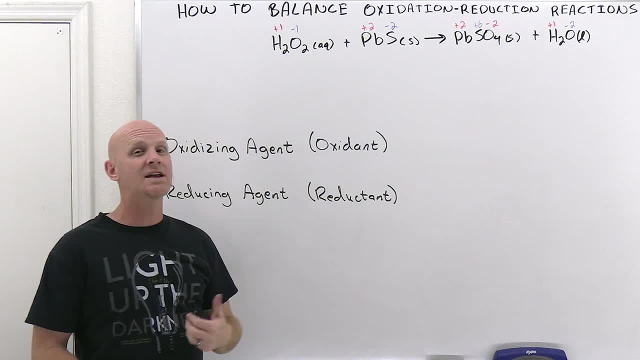 you could say the entire reactant species it's a part of. So you could also say that H2O2, hydrogen peroxide, is being reduced, And both of those are true statements. So, whether you want to identify the specific element within a compound, if it's in a compound, sometimes it really is in. 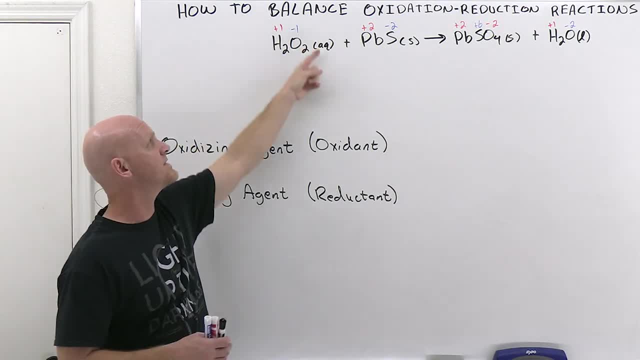 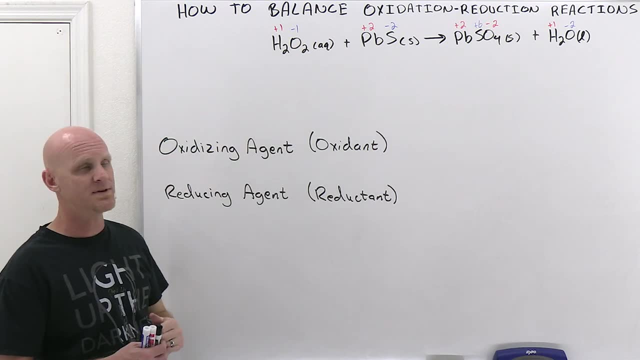 its elemental form and it's just the element. So, or whether or not you want to identify the entire chemical species- in this case compound- that it's a part of. either way, on the reactant side you can say it's the element or species being reduced. 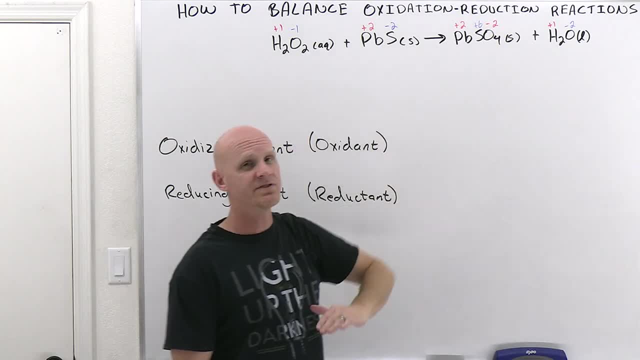 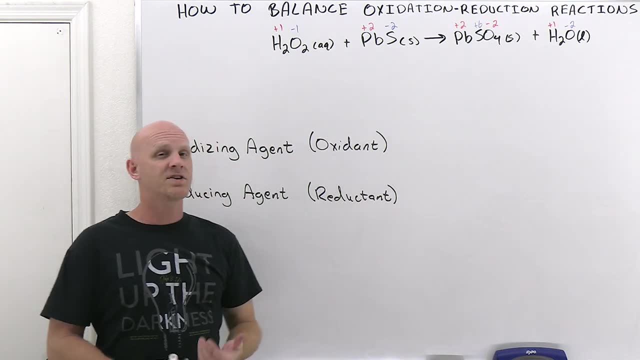 Now, if we look lead right here is plus two and lead's plus two. he's not changing either. But sulfur goes from minus two up to plus six. His oxidation state's going up. So notice, when the oxidation state goes down, like we saw with oxygen, that's when it's getting reduced. 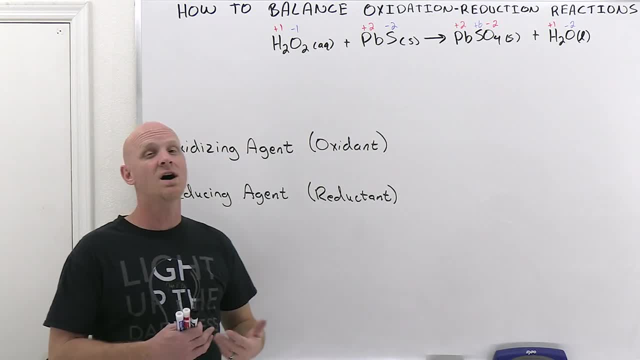 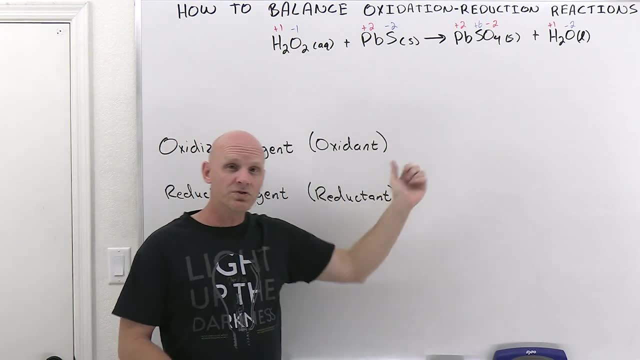 That's why they call it getting reduced. But when your oxidation state goes up, you're not getting reduced, you're getting oxidized, And this is where things get a little bit tricky. So oxygen again was getting reduced. But if you recall what reduced means, it means gaining electrons. 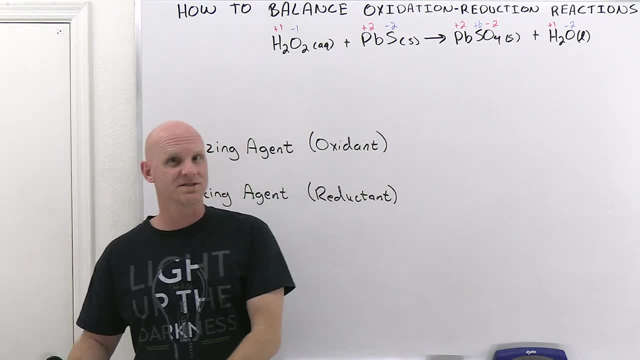 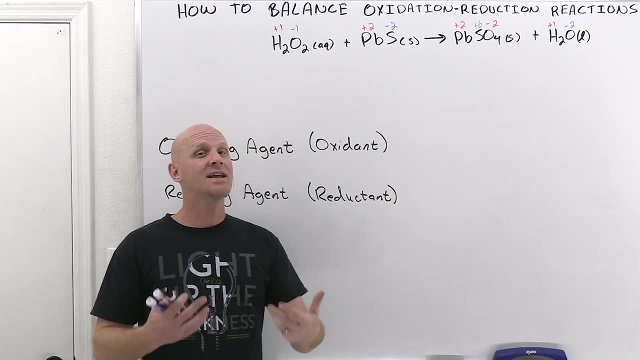 And notice we normally associate, you know, something being reduced with losing something, And you know it's all backwards because we're gaining or losing electrons which are negatively charged, And if you gain negative charges, your oxidation state goes down. 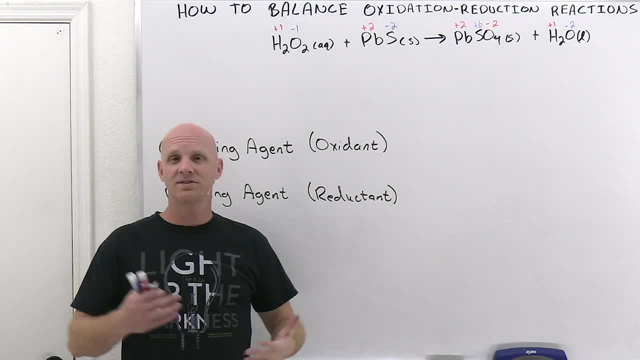 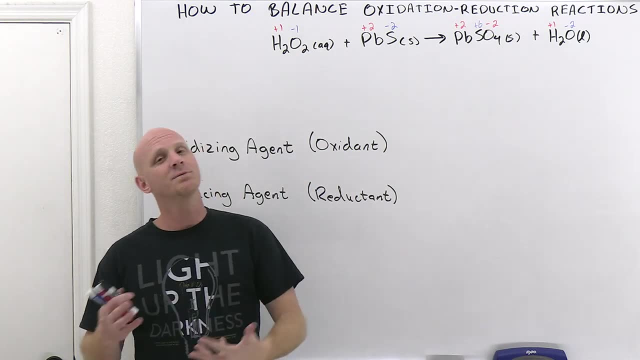 And if you lose negative charges, your oxidation state goes up. So exactly the opposite. if we think about it like with your bank account, If you lose money, your bank account doesn't go up, it goes down. And when you gain money, your bank account doesn't go down, it goes up. 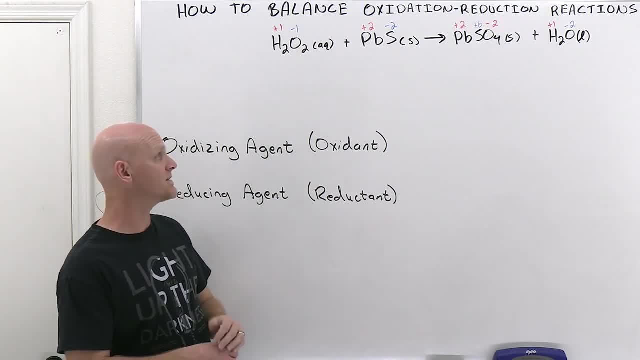 So. but it's all backwards when we're talking about negatively charged things, like electrons in this case. And so again key here- they call it reduction, because your oxidation state gets reduced, It goes down, but you're gaining electrons. So just kind of keep that straight in your head here. 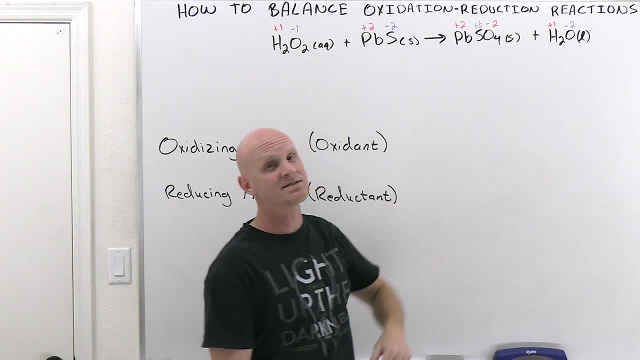 So, but in this case, sulfur going from negative 2 up to positive 6, it's definitely not going down. So it's not reduced, It's going up, That's being oxidized, That's a loss of negative charges, a loss of electrons. 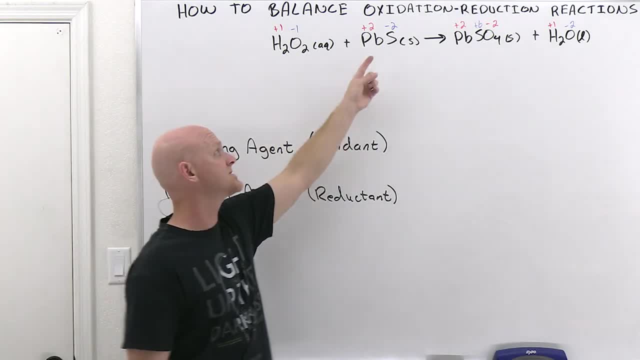 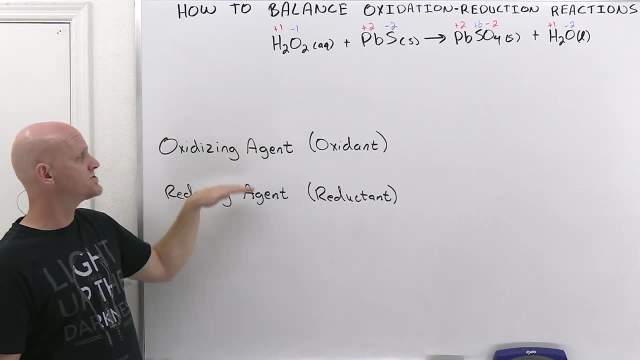 All right. Now, whether you want to say that sulfur was getting oxidized or that PBS was getting oxidized, both of those are true statements, And I'm emphasizing this for a point. We're going to introduce two new terms here: the oxidizing agent, or oxidant for short. 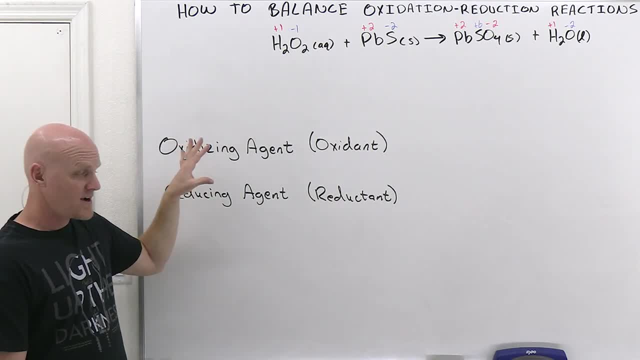 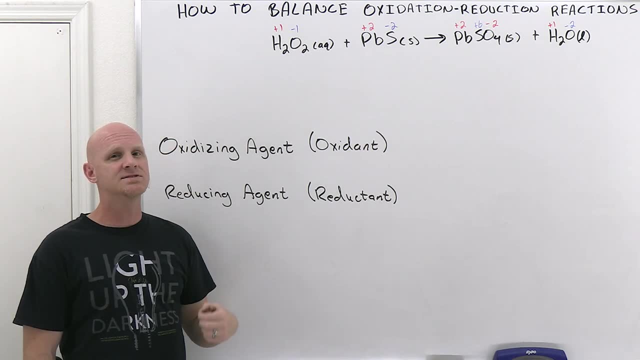 the reducing agent, or reductant for short. So- and these are going to seem a little bit backwards at first, but we'll be able to explain why that is- So it turns out, the oxidizing agent is the reactant species that is being reduced. 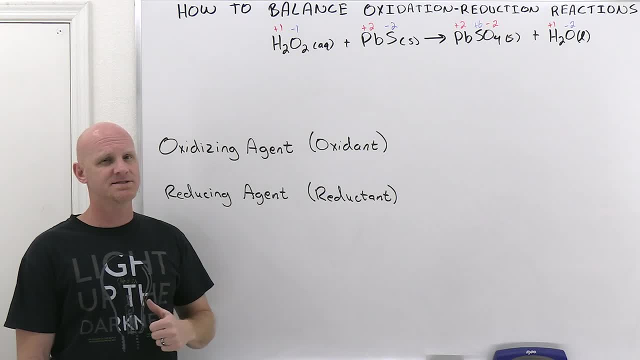 Okay, The reducing agent is the reactant species that is being oxidized, And this is going to seem backwards here for a second, So, but it has this terminology for a very specific region. So let's just say that you were sick of my videos and you came over to my house. 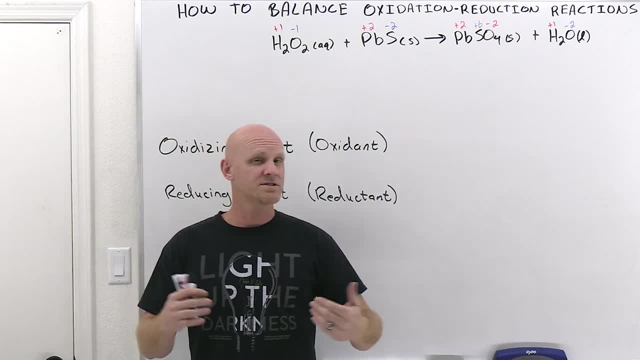 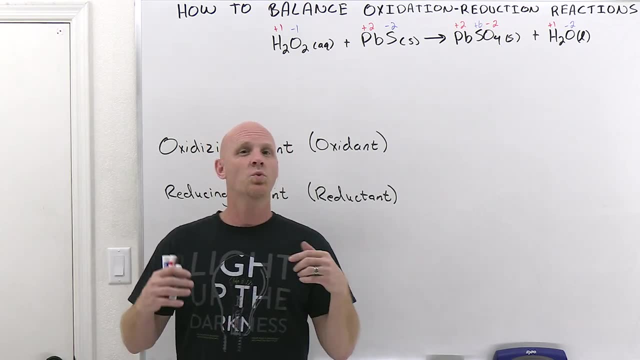 and you punched me in the face, And so my question for you is: who got punched? Well, I got punched, But did I do the punching? No, you did the punching, And so the one who does the punching and the one who gets punched are not the same person. 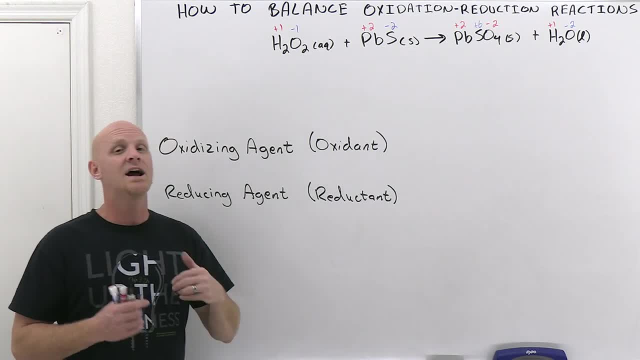 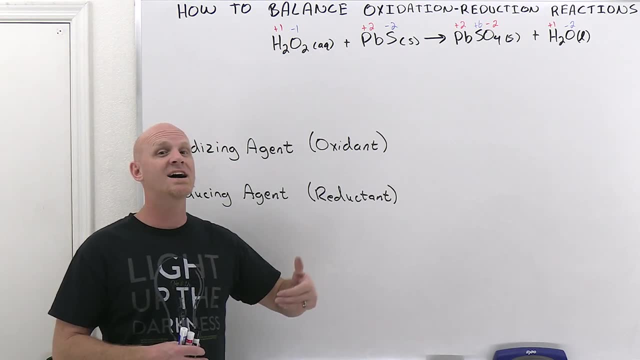 In the same context. here, the species that gets oxidized and the species that does the oxidizing are not the same species. The species that is doing the oxidizing is causing something else to get oxidized, Just like when you came over to my house and did the punching. 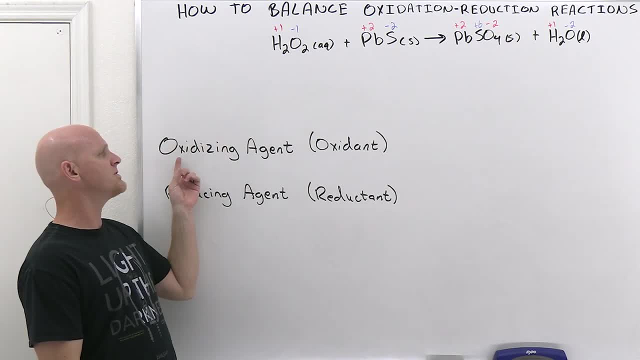 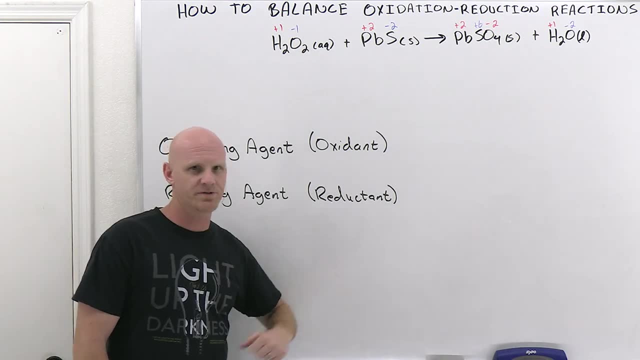 you caused someone else to get punched. So same thing here. The oxidizing agent is causing something else to get oxidized. It's kind of like the secret agent I've hired to steal electrons from somebody, but it's causing somebody else to lose electrons. 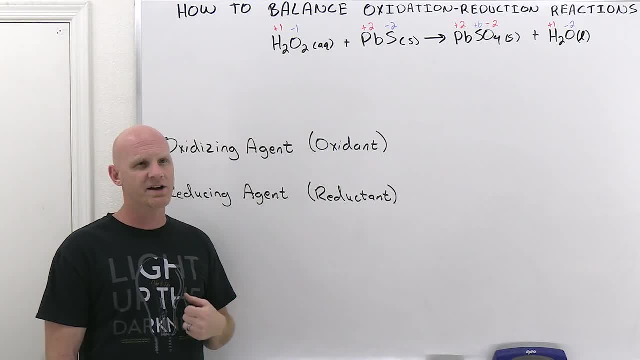 Well, how does the oxidizing agent cause another species to lose electrons? By taking them from them? And if the oxidizing agent is taking the electrons, well, that means the oxidizing agent is gaining those electrons and is therefore being reduced. So that's why the terminology seems backwards at first glance. 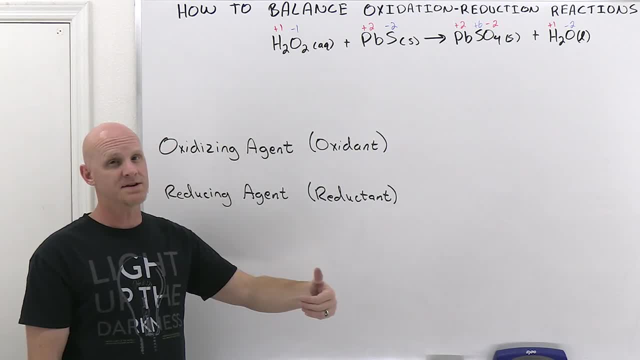 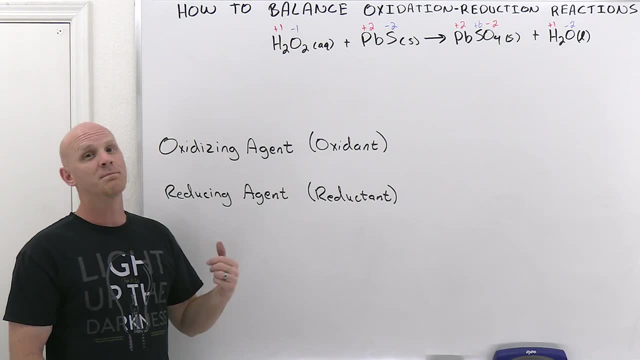 but they've got it correct here. The oxidizing agent causes another species to get oxidized by itself being reduced, and the reducing agent is going to cause another species to get reduced by itself being oxidized. All right, so if we go back and look at this, 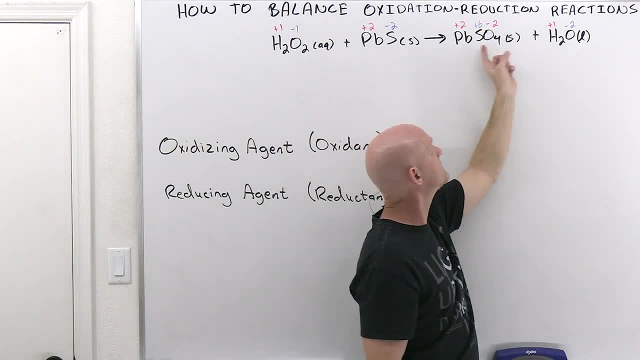 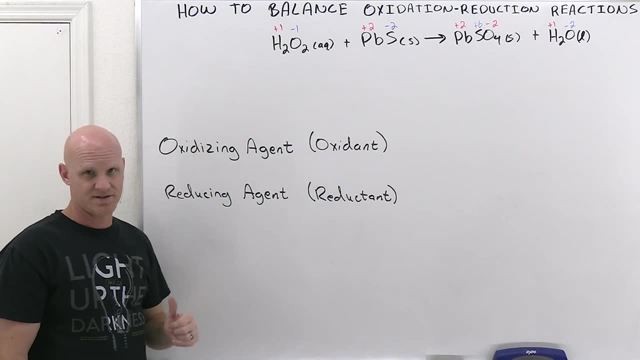 we said here that oxygen was going from minus one to minus two, no matter how you sliced it, and he was getting reduced. Well, the species that gets reduced is the oxidizing agent. However, we have to be a little bit careful. 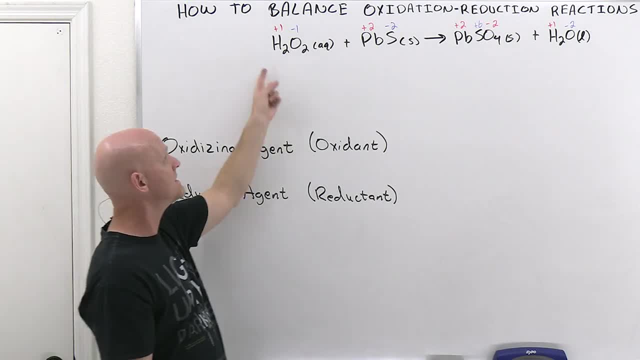 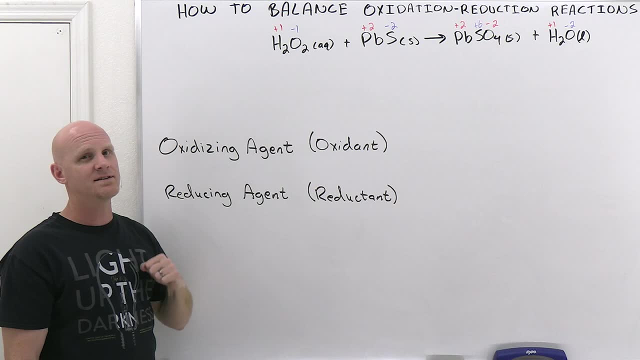 We said that we could say that it's the element, oxygen that's getting reduced, or we could said that it's hydrogen peroxide, H2O2, that's getting reduced. But when you identify the agents here, you have to name the entire reactant chemical species that that element is a part of. 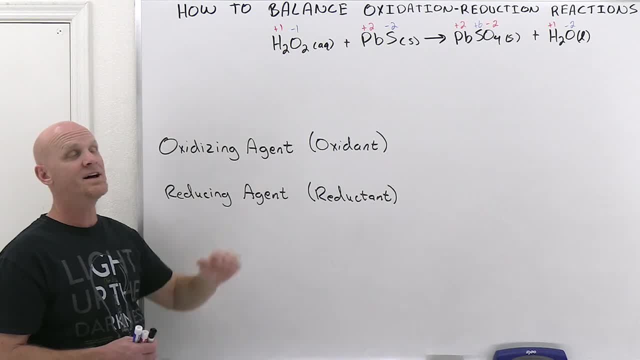 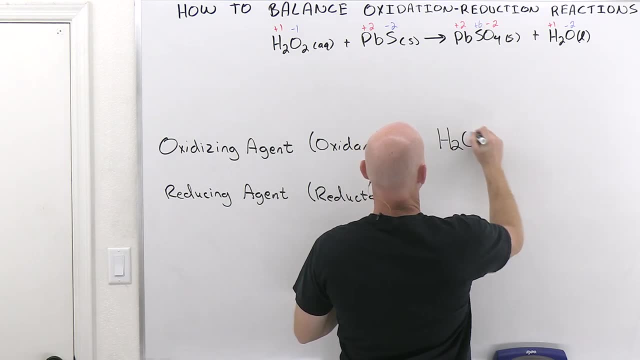 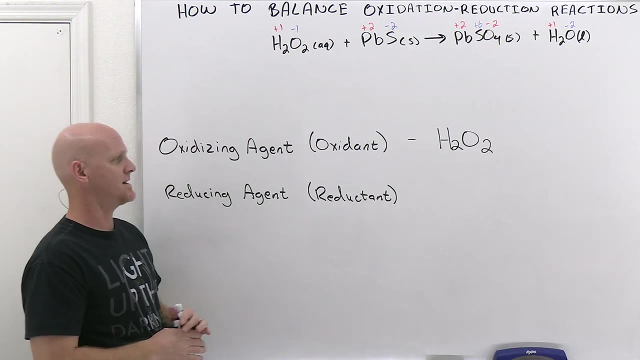 So you couldn't say that oxygen, in this case, is the oxidizing agent. You'd have to say that hydrogen peroxide, H2O2, is the oxidizing agent. So be careful: When we identify these agents. it's the entire chemical reactant species that we have to identify. 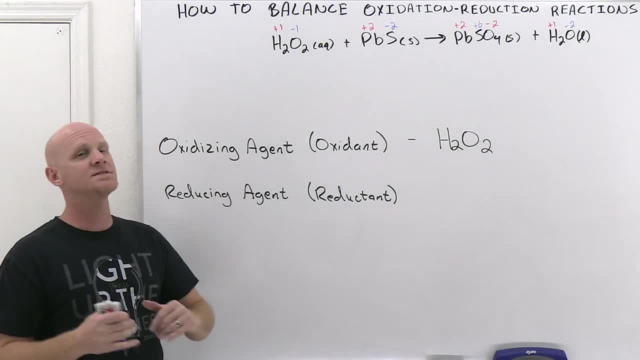 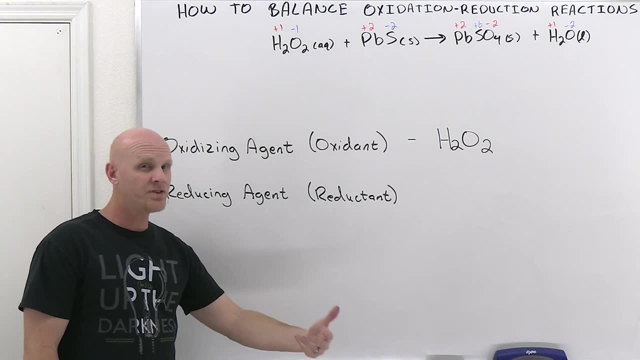 not just the individual element, unless it happens to be in its elemental form, but otherwise it's the entire chemical species, either compound or ion. So the reducing agent? well, the reducing agent is causing something else to get reduced, It itself is being oxidized. 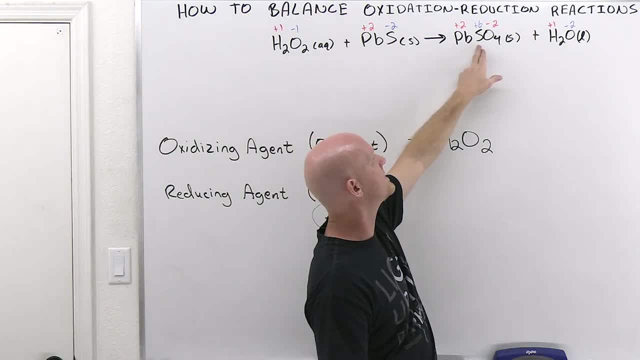 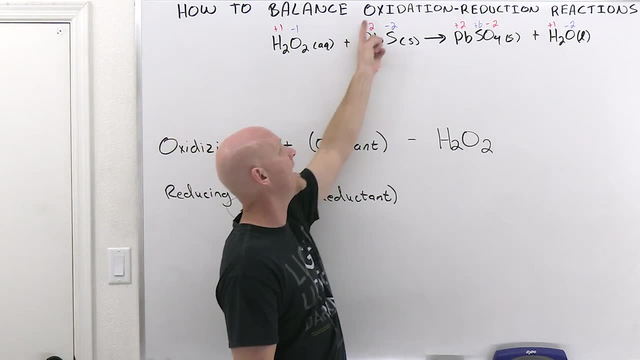 It's losing electrons. So when we identified that, sulfur was the one that was losing electrons getting oxidized. but again, if I'm going to name the agent here, the reducing agent, I can't just name sulfur, I have to name the entire reactant species he's a part of. 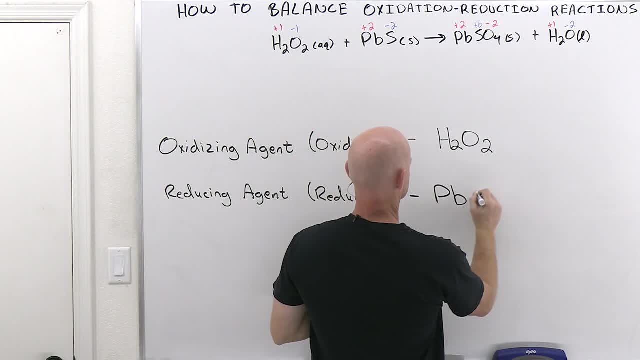 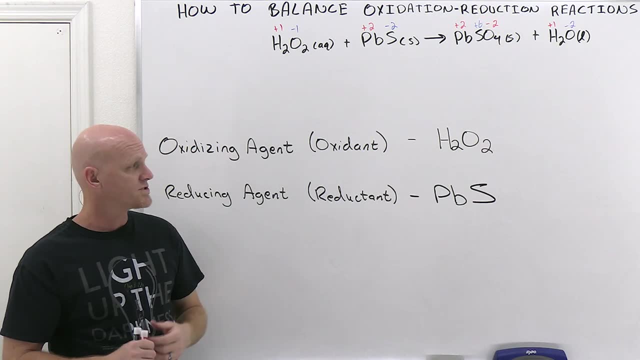 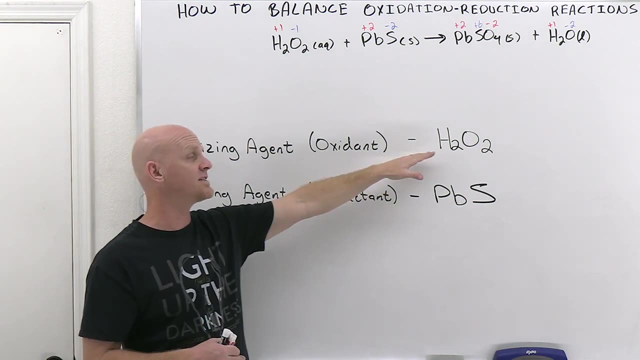 which is PBS. And so PBS here is the reducing agent, or reductant for short, Cool. So I just want to make sure you realize first of all how we define oxidizing agent, reducing agent, how to identify them and then properly how to identify that it's the entire chemical species. 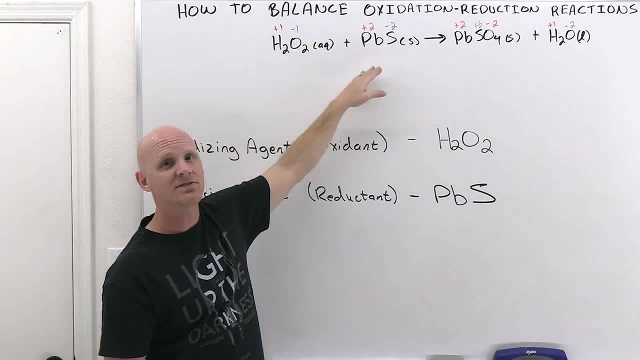 Notice: the agents are always, always going to be on the reactant side of a reaction, never on the product side. Where do the whys? Also, the species getting oxidized and reduced are also always going to be on the reactant side. 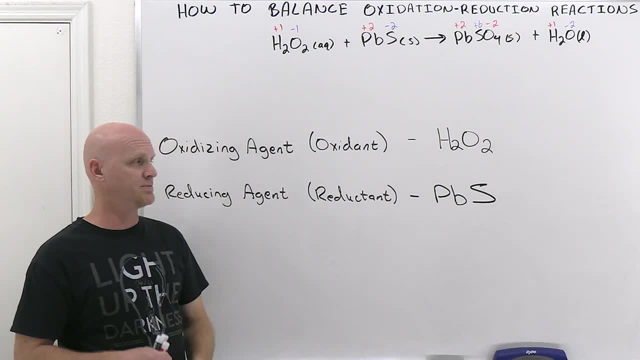 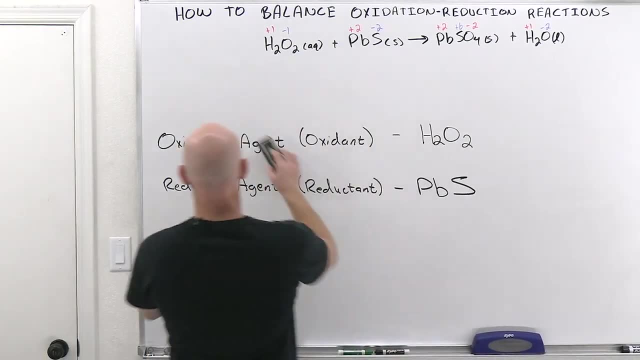 never on the product side, If you're, at least if you're identifying the entire chemical species. just keep that in mind. All right, So now that we've got through that, let's go back to balancing these lovely redox reactions. So with the half reaction method, 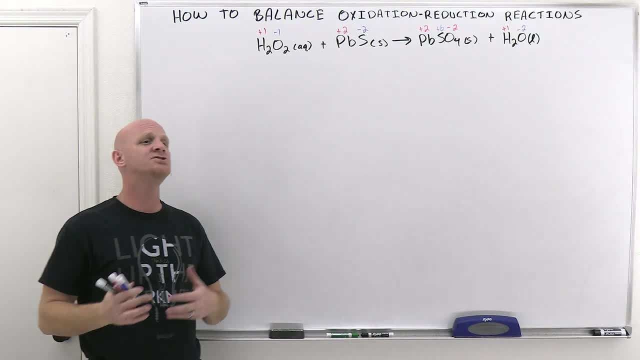 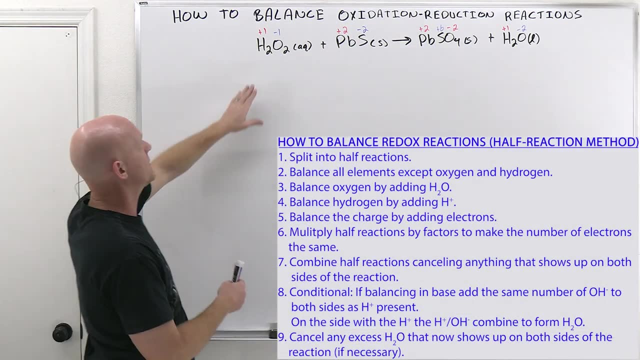 and so it turns out we're going to split apart the oxidation half of the reaction and the reduction half of the reaction into separate what we call half reactions, and that is going to be the first step in this half reaction method. So in this case, 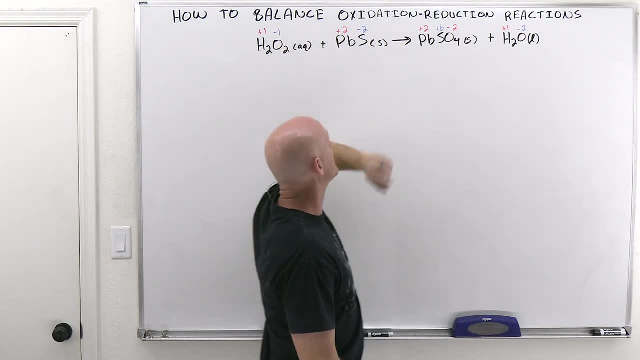 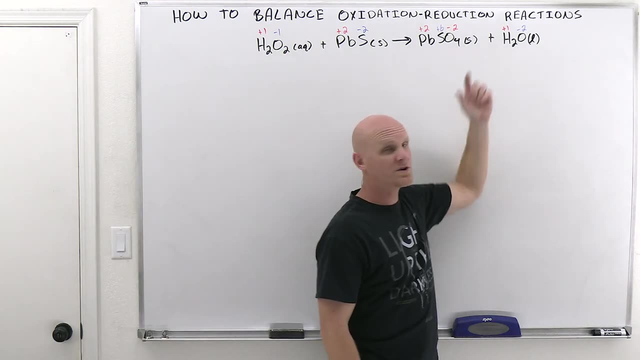 we can look at oxygen going from negative one to negative two, So, and then sulfur going from negative two to positive six, and it might be a little unclear. Well, is oxygen negative one to negative two, either here or here? Which one is it? 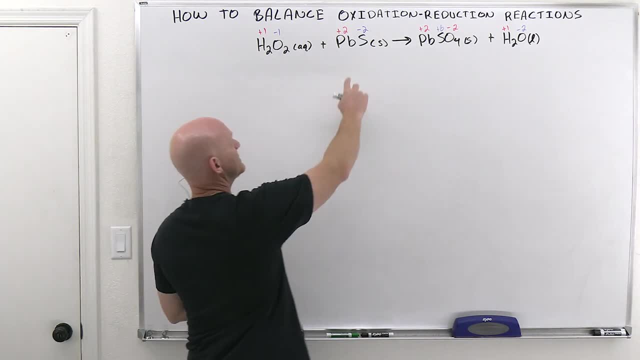 Well, we'll come back to that in a sec. Let's do the other half first. It's a little bit easier to identify. Sulfur only has one place to start and one place to end up, and that has to be one half of the reaction. 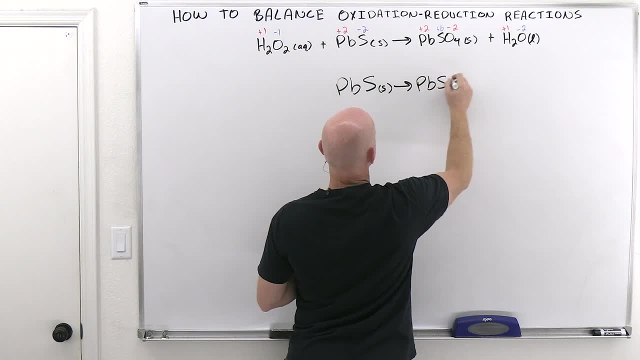 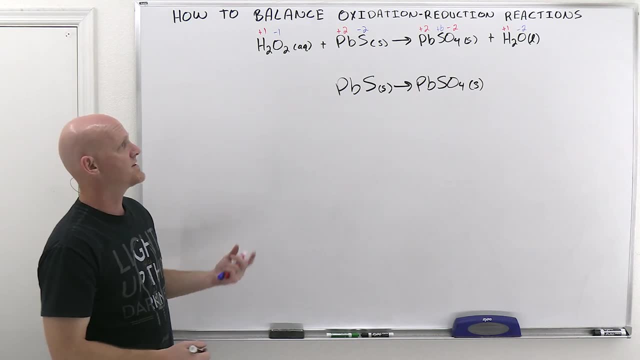 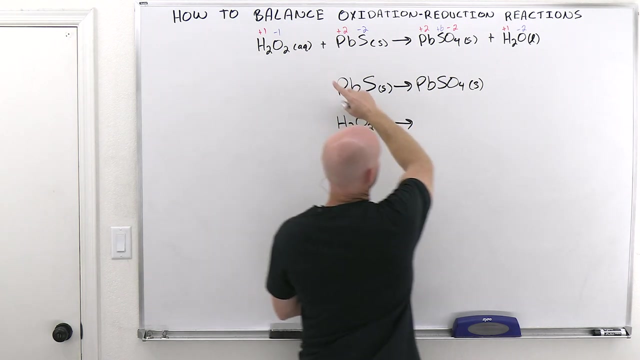 So if PBS solid going to PB, SO4 solid and that's going to be the oxidation half of the reaction, All right, So then what we got left, then H2O2 definitely involved And therefore is going to have to be involved with water on the other side. 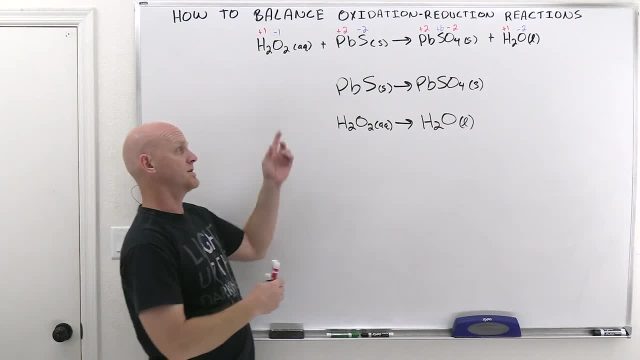 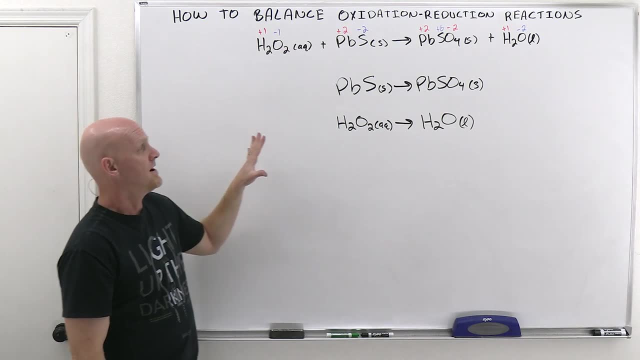 The thing we haven't used yet. So technically we could have thought: well, maybe it's going to be with the auctions and the PBSO4, but we already used them in the oxidation half, So it'll just be the oxygen, the water and the reduction half here. 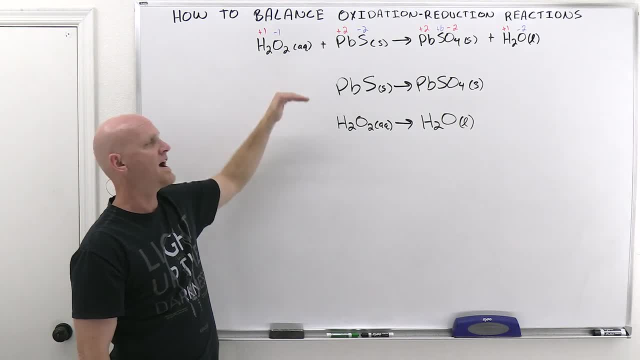 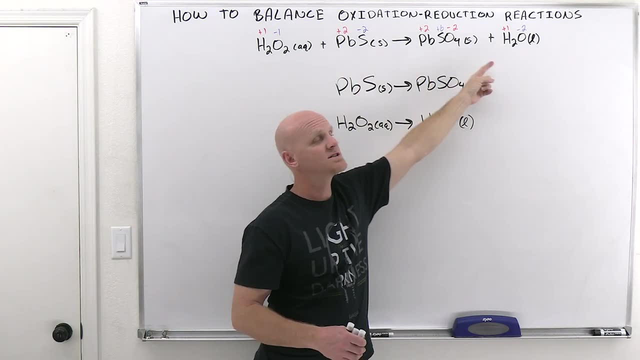 All right. So now we split this up Into half reactions and oxidation half and a reduction half. And no, we might not have realized this was the oxidation half And this was the reduction half, Had we not already assigned oxidation numbers. So, and the truth is, you don't actually have to start off by assigning oxidation numbers. 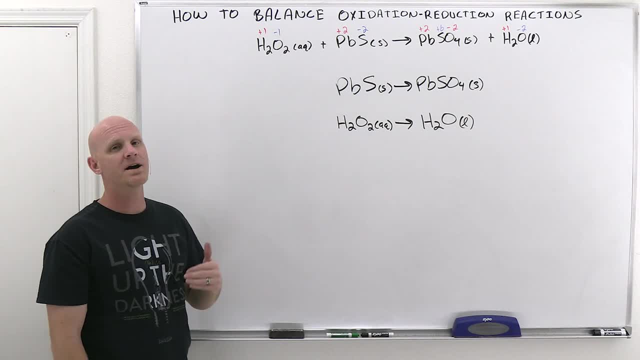 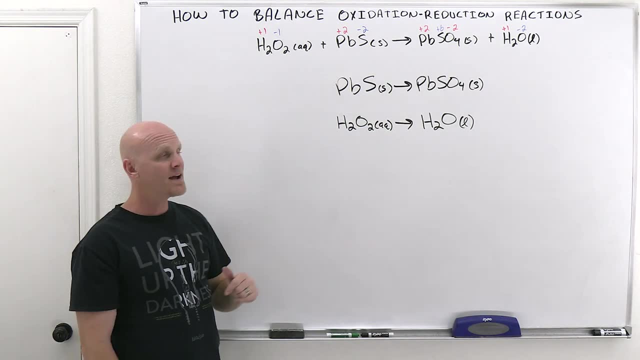 In fact that's going to slow you down quite a bit. As long as you can identify who's oxidized, who's reduced or at least who's going to be changing oxidation states and put them in separate half reactions, I wouldn't even care if you knew this was the oxidation half. 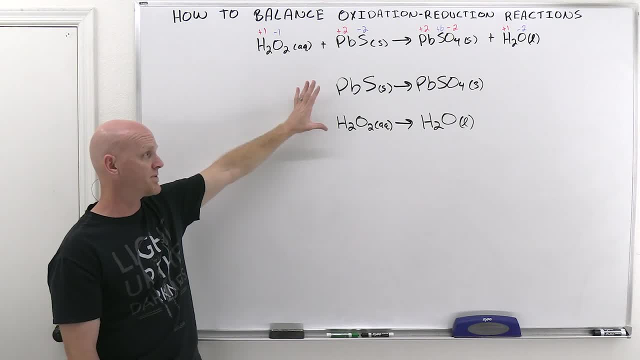 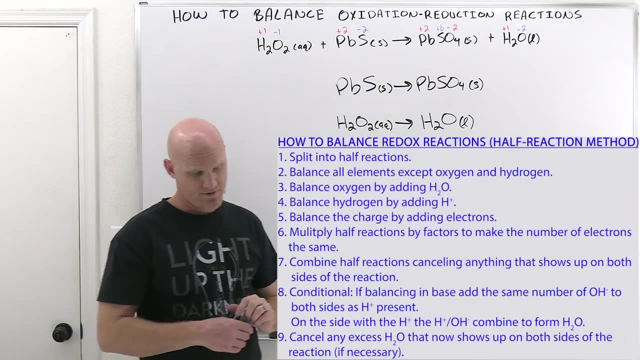 and this was the reaction- half. just as long as you properly identified the two halves and split it up, Good place to start. All right, So now you want to balance all the elements except for oxygen and hydrogen. So it turns out we're going to balance oxygen and hydrogen in a special way. 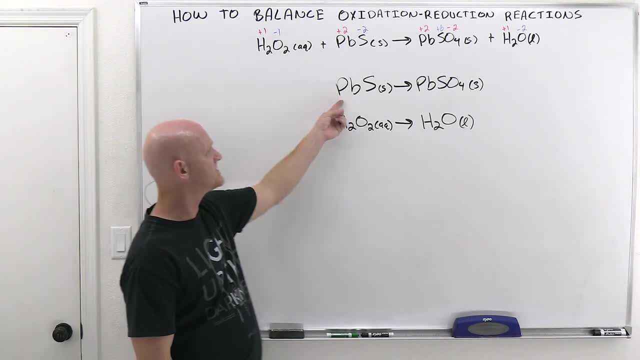 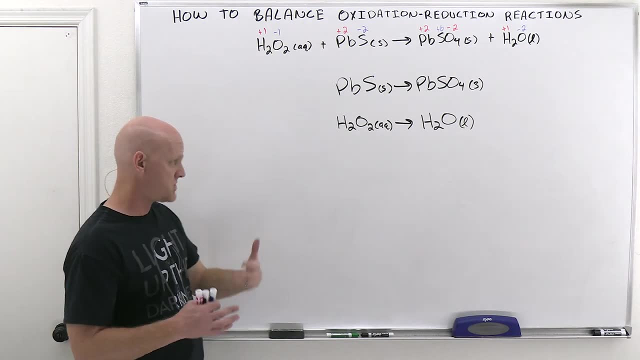 So you want to balance all the other elements first. So, in this case, want to make sure the leads are balanced. They are want to make sure the sulfurs are balanced, They are. the only thing not balanced is oxygen, and you always save oxygen and hydrogen for last. 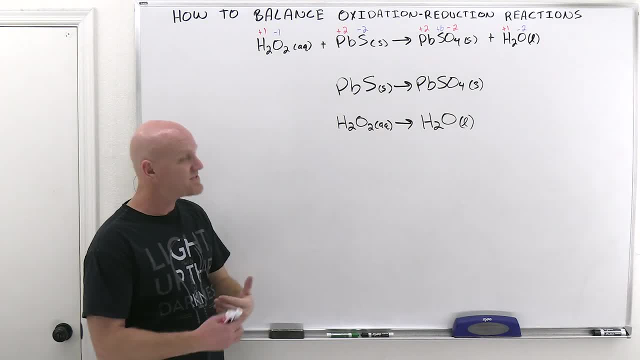 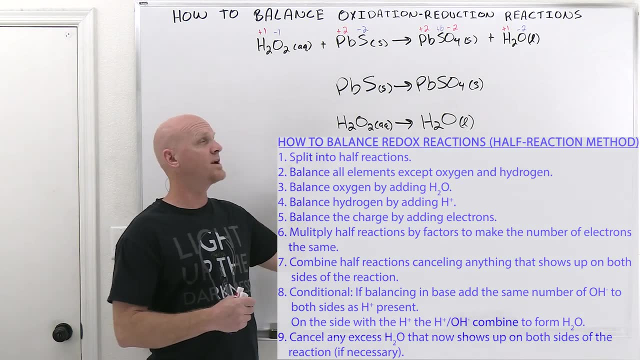 Okay, and the other half? all we have is oxygen hydrogen, So everything else is already balanced, All right. so that's rule number two. rule number three: Balance oxygens by adding water. So it turns out our Redox reactions are always going to be aqueous. reactions are taking place in water. 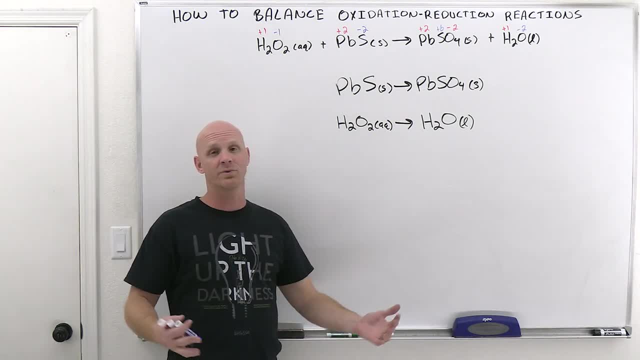 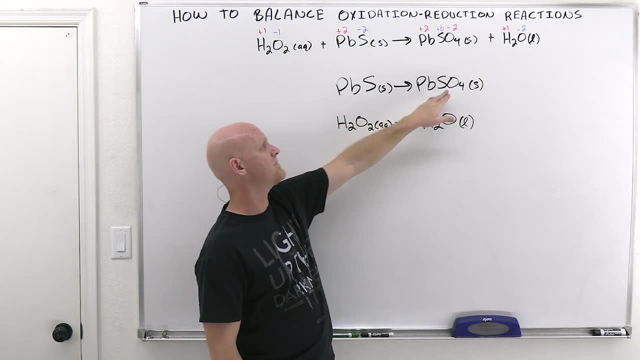 And so water has the option of showing up as a reactant or product in any given Redox and it turns out. that's why we're able to balance auctions by adding waters. in any case, Now in the first half, the oxidation half, we've got four auctions on the right. 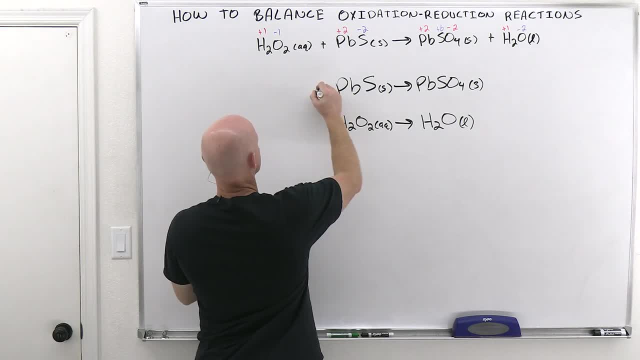 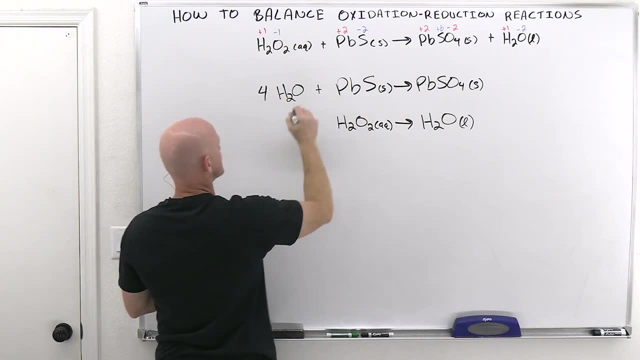 We don't have any on the left, So we're going to need to add some waters over here. and the question becomes: well, how many waters? well, in this case, I got four auctions over here. I need to have four oxygens over here. 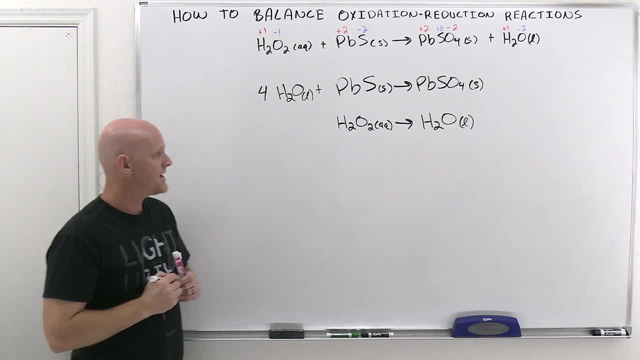 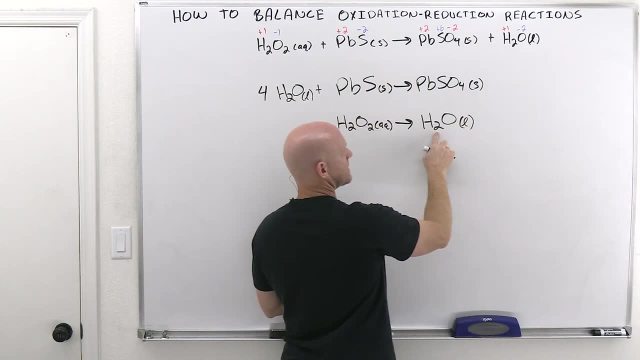 So we'll have to add four waters in the other one. here We've got two auctions on the left, one auction on the right, So we'll have to add another water over here and instead of putting plus water- Well, this is water as well. 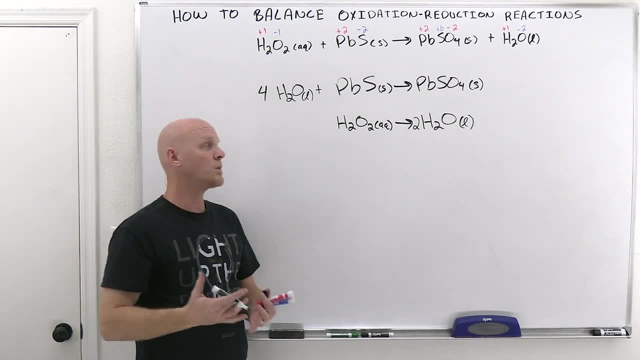 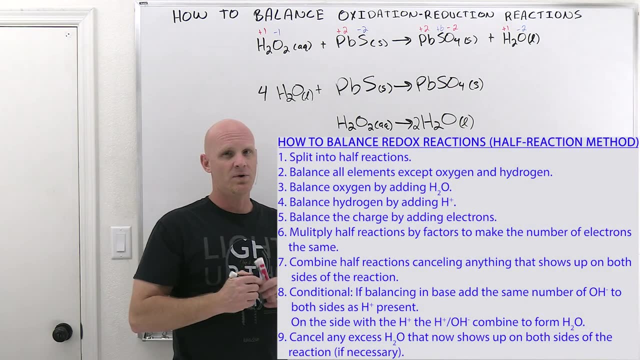 I'm just going to put a two here. It's not normally how it work, because we don't normally already have water in the in the half reaction, but we did in this case. All right. Finally, now we balance hydrants. Now we always do auction second to last and hydrants is the very last thing you balance. 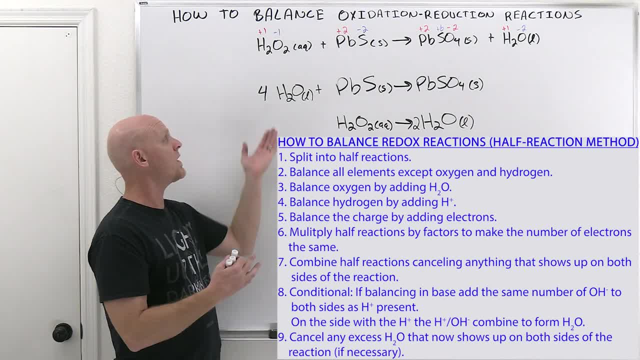 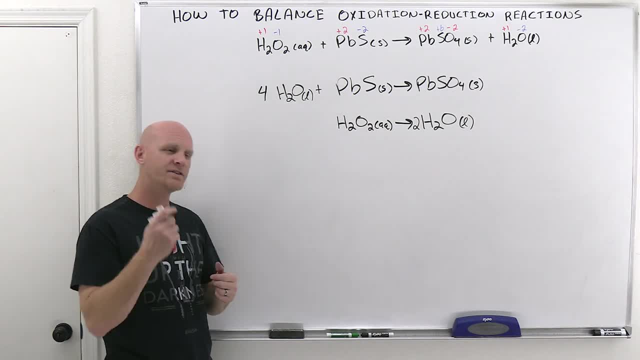 and the reason that is is that, well, you balance auctions by adding waters, and when you add water you're going to add more Hydrogens, and if you'd already bounce the hydrants first, well then that would throw it off. So it's always auction second to last and hydrants very last. 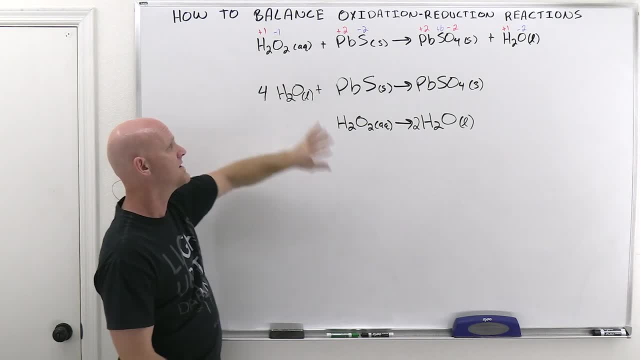 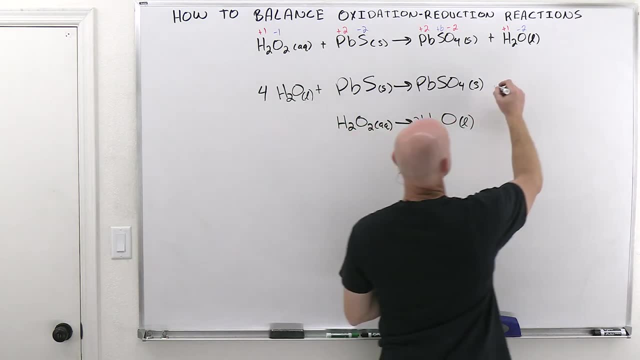 and in this case we've got a total of eight H atoms on the left, So we're going to need eight H atoms on the right. and just like we always balance auctions with by adding water molecules, We're always going to balance hydrants by adding H plus. 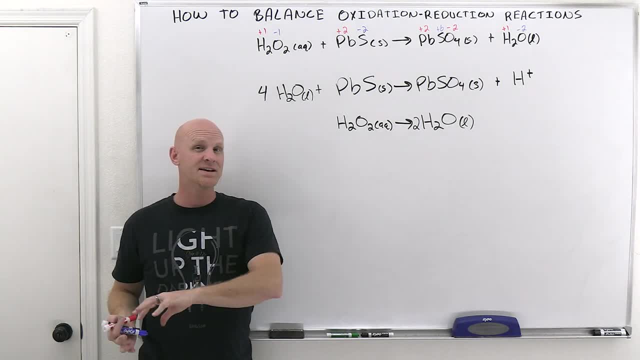 Cool. Now it turns out that Redox reactions can happen either under acidic or basic conditions. The evidence that they're under acidic conditions is H plus. the evidence that they'd be under basic conditions would be the presence of OH minus. So and it turns out by default with our half reaction method. 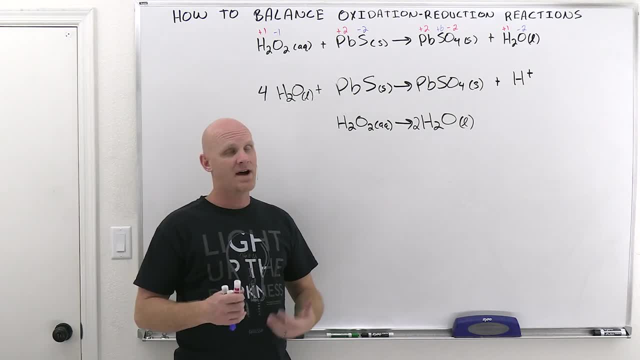 We will always, by default, balance in acid, and if you have to balance under basic conditions- and you'll find out that you can be asked either- then we'll have an extra step to add at the very end. But by default we'll start always by balancing an acid. 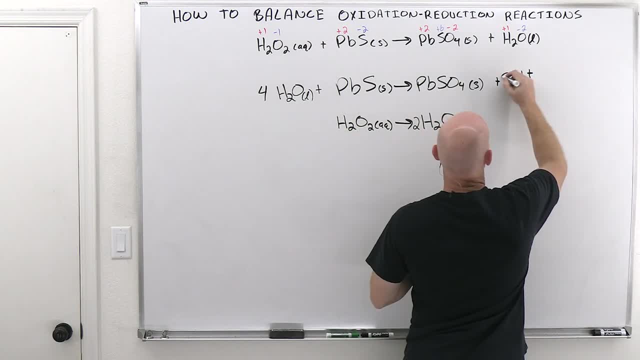 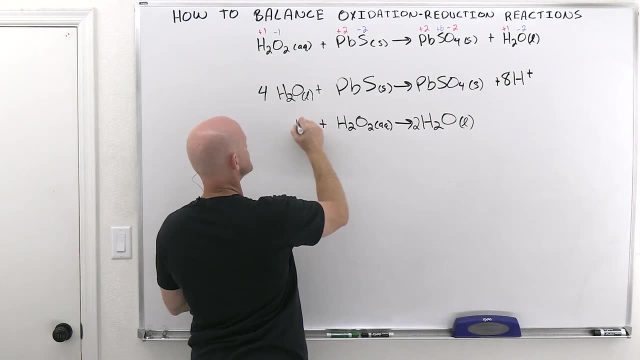 All right Now. we've got eight H's over here, So I'm going to need eight Pluses here for this one. We've got two ages on the left. We've got a total of four H's on the right, So I'm going to need more H's on the left. 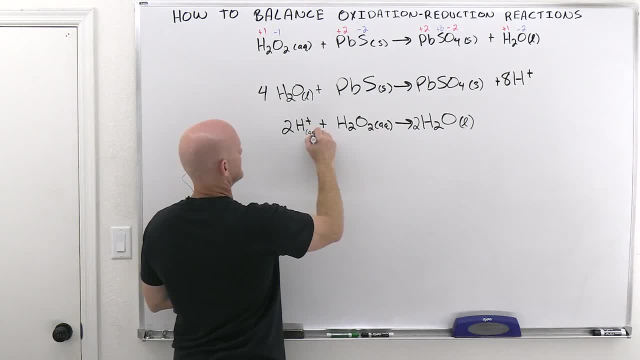 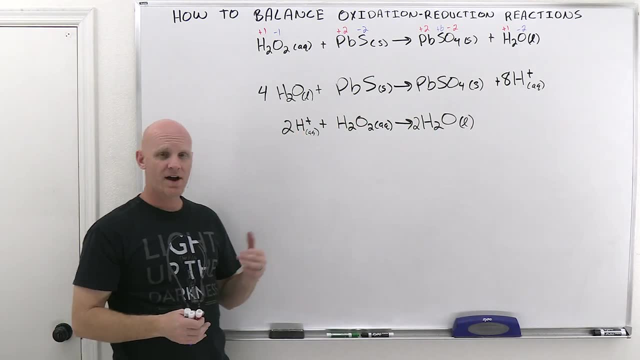 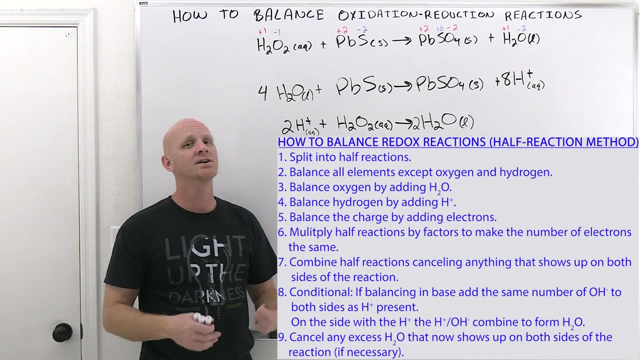 And in fact I'd need two more. Let's get some States on there. And now all the elements are balanced. So again, oxygen second to last, hydrants dead last. and once all the elements are balanced, you see that rule number five says: balance the charge by adding electrons. 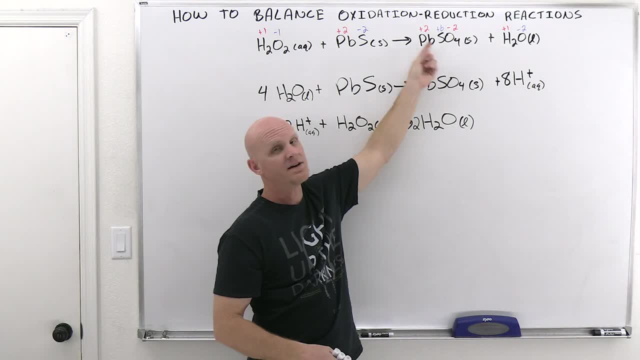 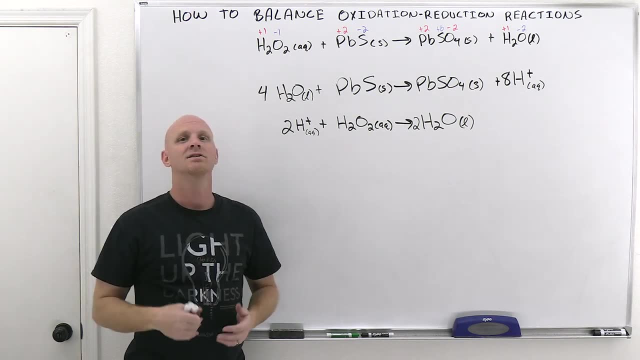 Now you might look at this and be like: well, sulfur went from minus two to plus six, That's a change of eight. all the way down, you know, two below zero to six above zero, That's a change of eight. So, and we might figure out that all that today, eight electrons being lost. 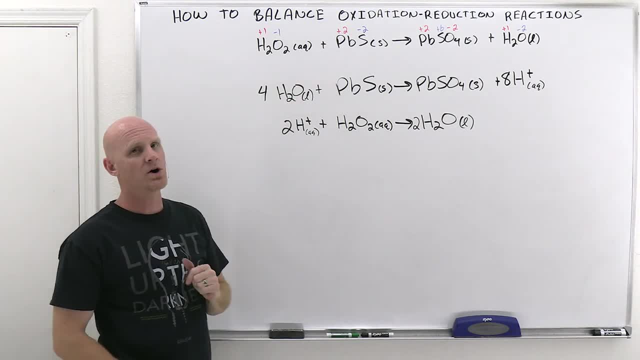 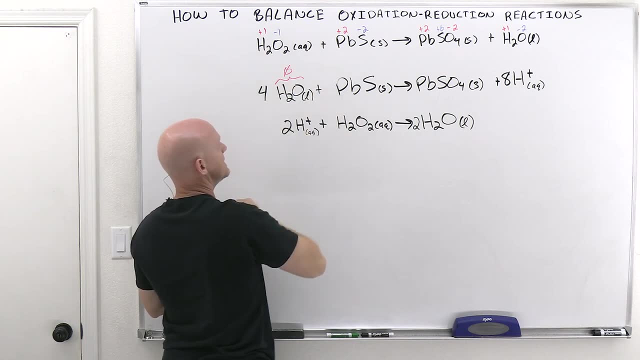 So, however, we don't need to figure that out. If we just balance out the charges overall here, we'd figure that out anyways. So if we look here, water is a neutral compound. I don't have to sign individual oxidation States, but as an entire compound, no overall charge. same thing with lead sulfide. 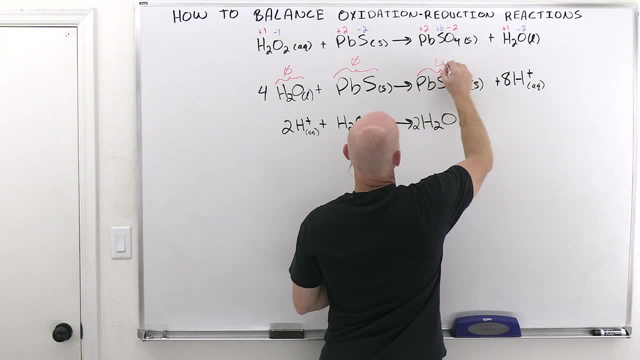 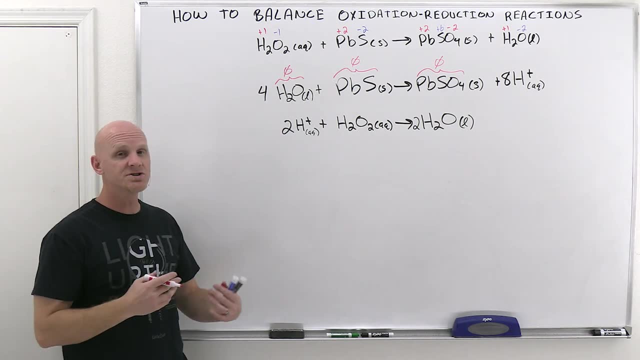 That's a neutral compound, No overall charge. and same thing for lead sulfate. That's an overall neutral compound, No overall charge. So I don't actually have to sign individual oxidation States for this purpose, Just have to know what the overall charges are on each side of the reaction. 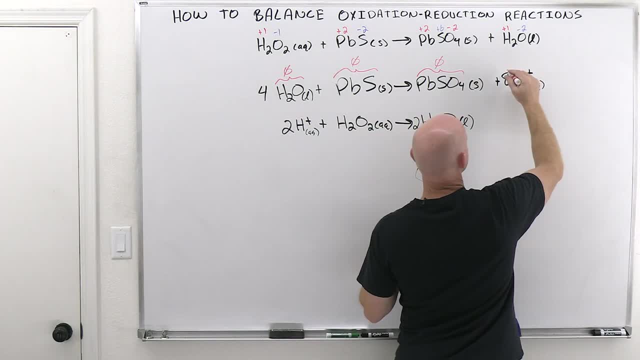 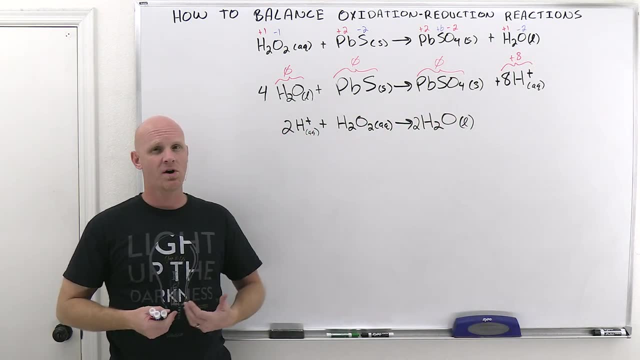 And so here we can see, though, that with eight H pluses there, plus one each, and there's eight of them, There's a total charge here of plus eight, And so now I need to add the electrons, and the electrons are going to balance out the charge. 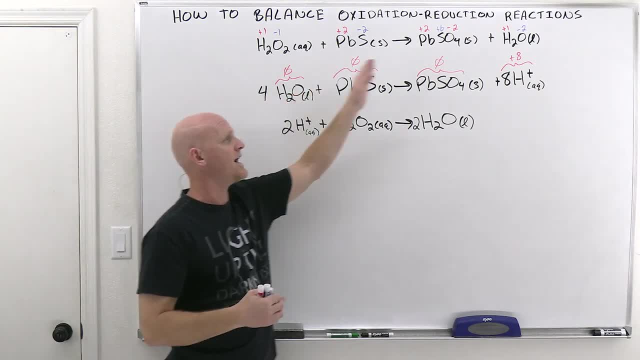 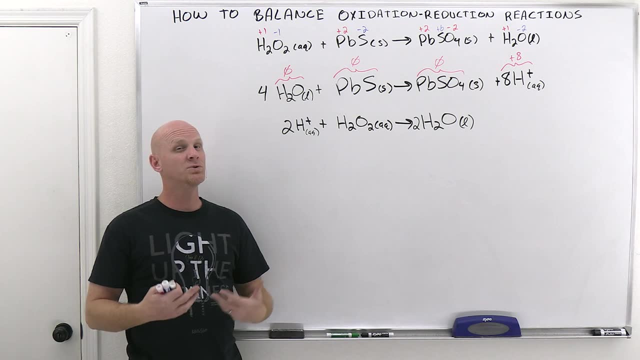 and since electrons are negative, you have to add them to whichever side of their half. reaction here is more positive: till the charges are the same, and it doesn't mean you, they have to both be equal to zero, but just till they're the same, if that happens to be zero. 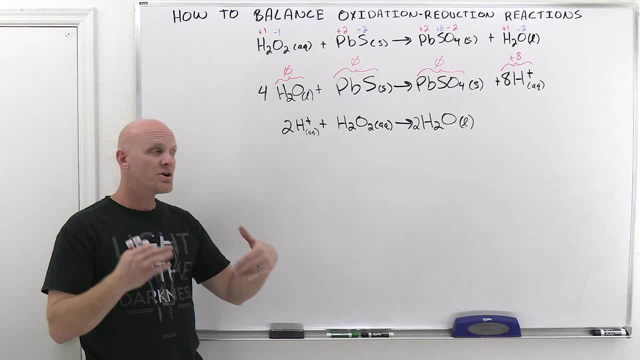 Great if it's plus two, great if it's minus two, whatever, just till they're the same. Well, in this case, this side is zero. this side is plus eight. This is the more positive side. It's the side that's going to get electrons. 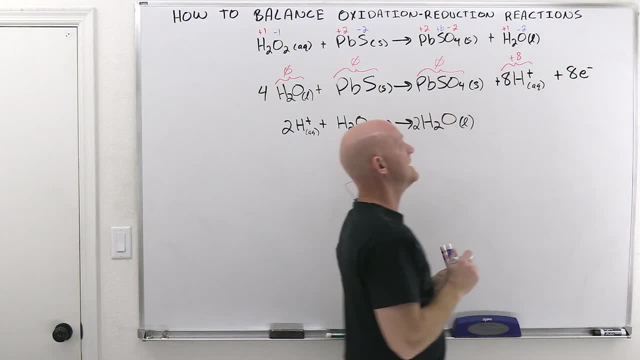 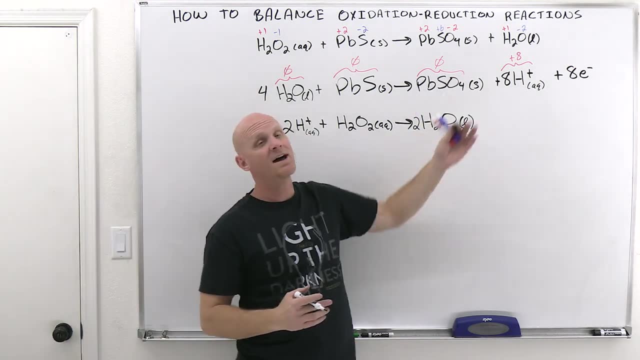 How many does it need till both sides have the same charge? That's eight electrons. now both sides would be zero. So, and it just happened to be because this side was already zero, But again, had this side been plus two, Well then I would have only added six electrons, or something like that. 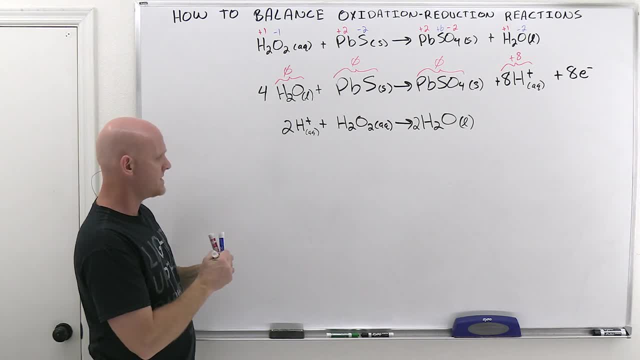 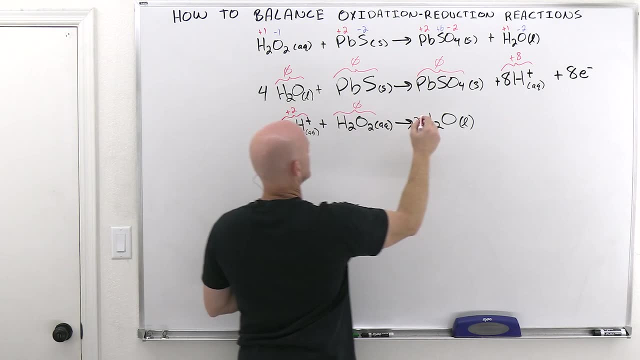 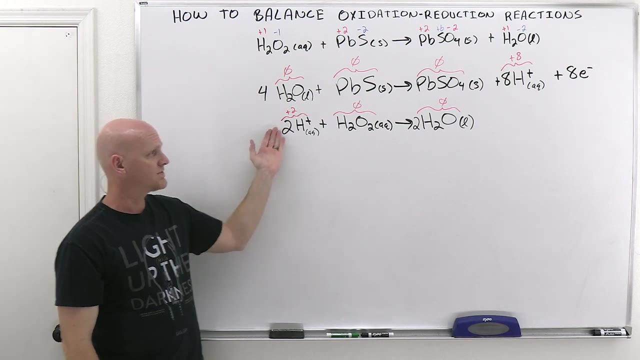 So, but the electrons balance out the charge. and the next one. here We've got a Total of plus two Right here. So but zero here And zero here, And so the more positive side now is on the left hand side It's plus two, the other side zero. 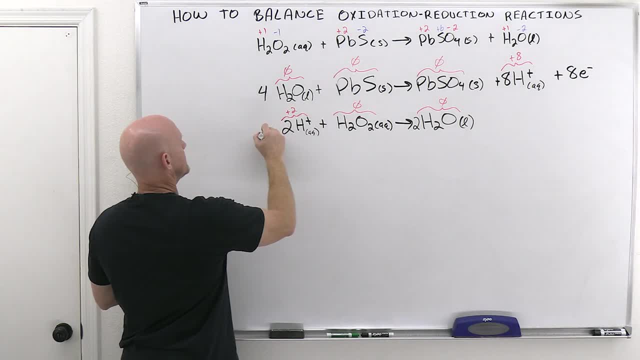 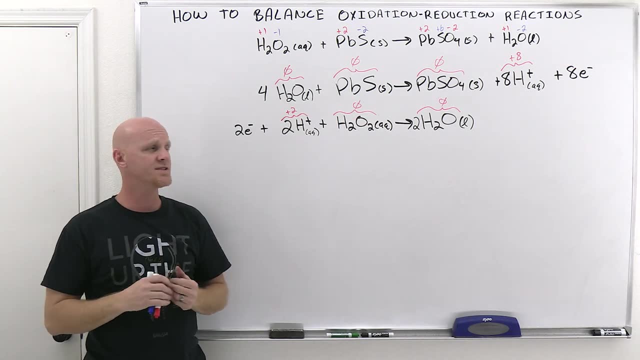 How many electrons do I need to add to this more positive side till they have the same charge? Well, that's going to be two electrons. cool. Now both sides have the same charge, and again it just happens to be zero in this example. 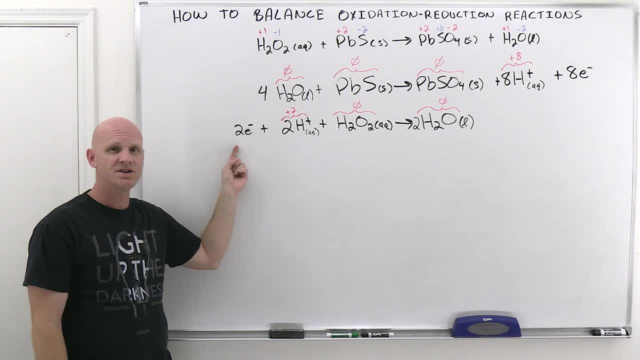 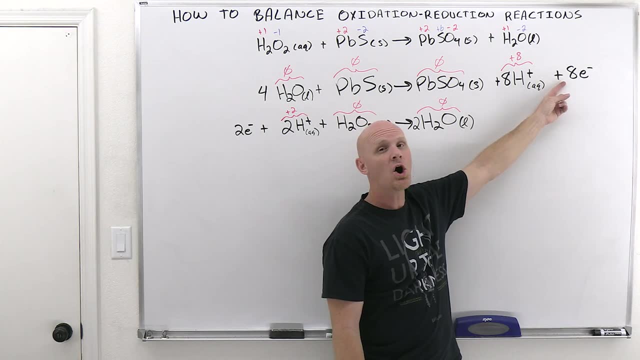 Now, when electrons are on the reactant side of the half reaction, that is the reduction Half reaction- Those electrons are being gained. when electrons are on the right hand side, the product side of the half reaction, Those electrons have been lost. That is the oxidation half reaction. 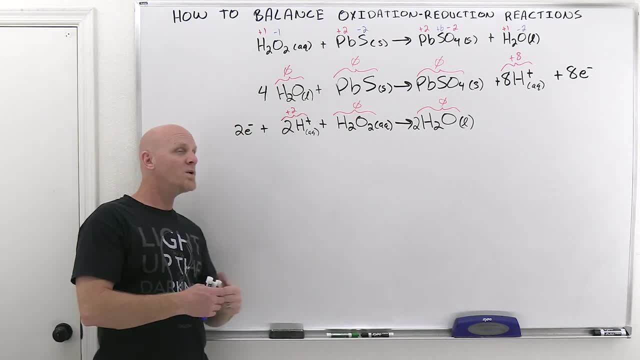 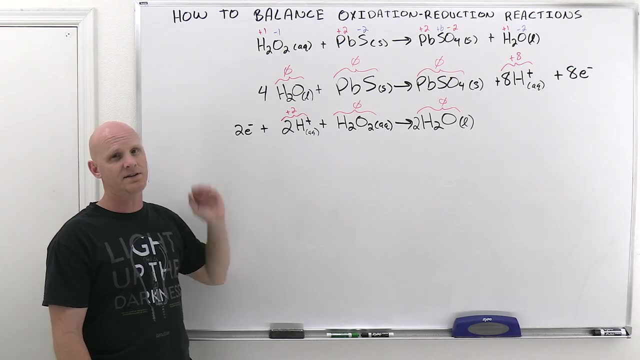 And again, if you've done this correctly, you should have electrons on one side and one half, and on the other side and the other half. This is an electron transfer reaction. We need no one species to have lost electrons and one species to have gained electrons. 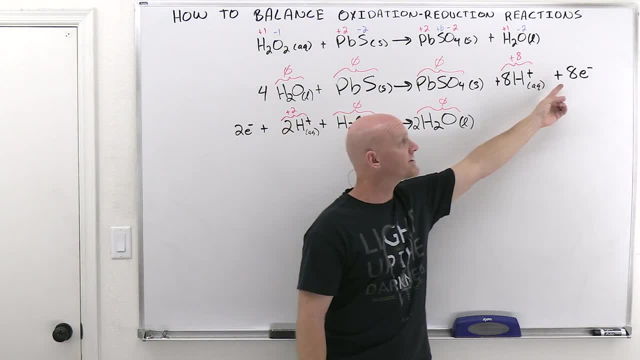 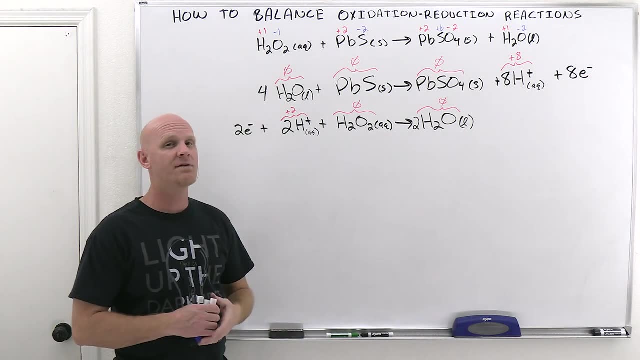 Now it turns out that the electrons that are being gained by one half reaction are the same electrons that were being lost by the other. It's just an electron transfer reaction, And so the number of electrons in both the half reactions has to match. So I can't just you know. 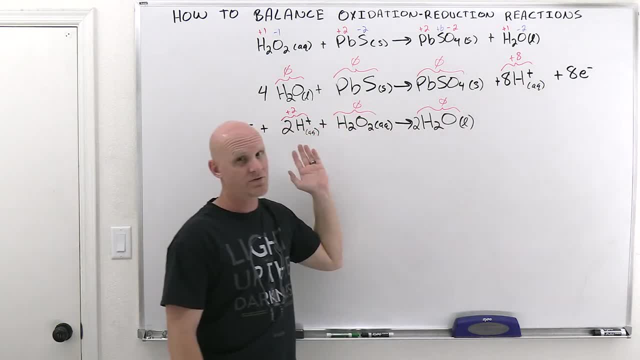 gain two electrons If I lost eight over here. if you lost it over here, you got to gain eight over here. So or if I gained two over here, I'd wanted to lost two over here. but these numbers don't match. 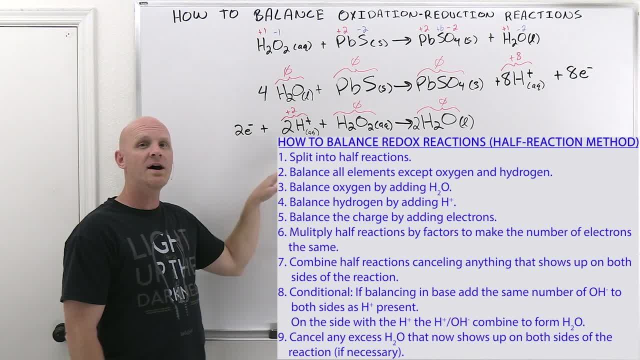 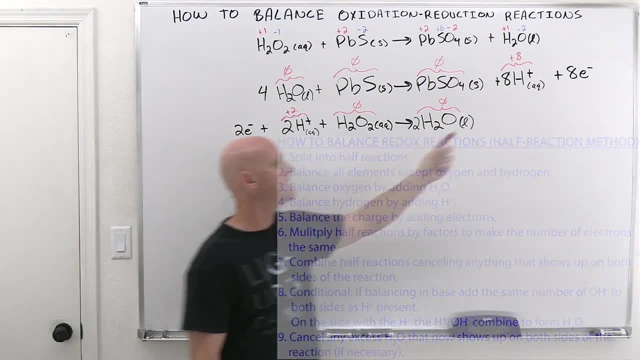 And so what you've got to say, then, is they need to match, and you need to multiply these by some multiples till they do match. And so the question you have to ask yourself is: what is the least common multiple between two and eight? And that's what you're going to balance it to. 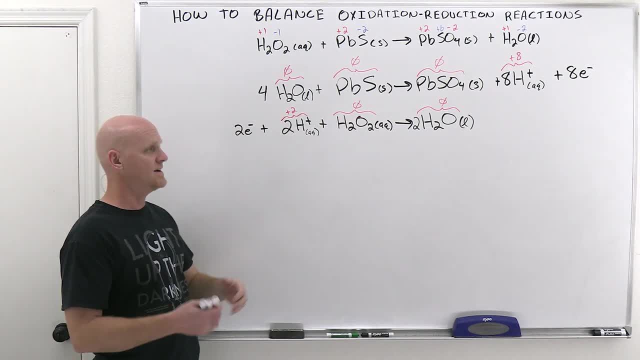 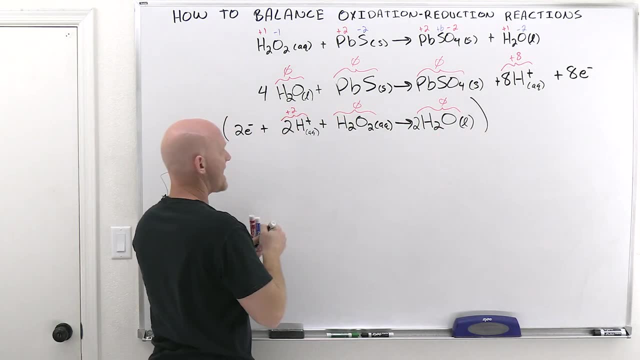 Well, the least common multiple between two and eight is eight. They both go into eight evenly, And so this one already is eight. I'll leave him alone. But this one is not eight yet, So we're going to go ahead and multiply this entire half reaction times four: 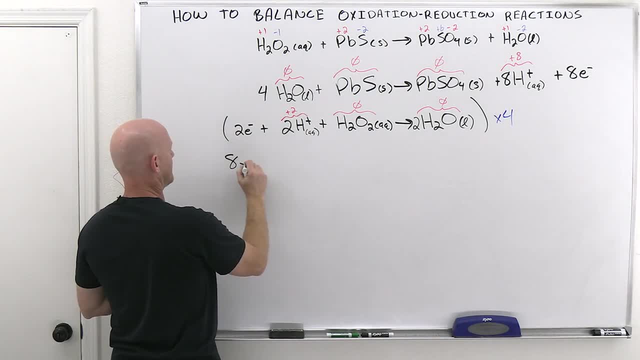 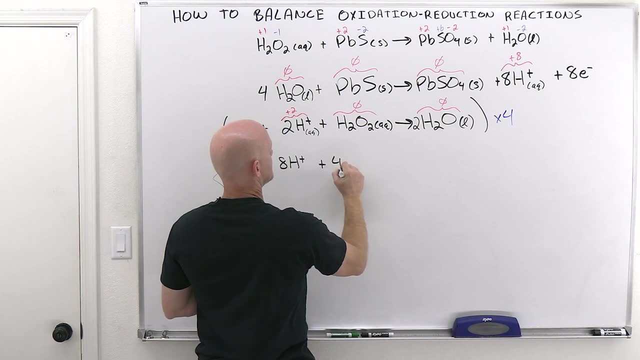 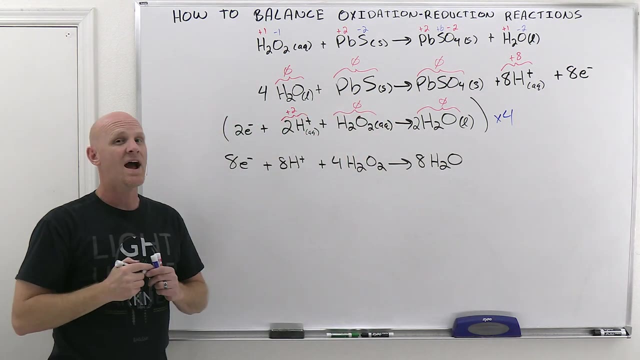 Cool And if you notice, that's going to make this now eight electrons plus eight H plus It multiplies all the coefficients by four plus four, H2O2 goes to eight H2O. So that is the new half reaction balanced out to eight electrons. 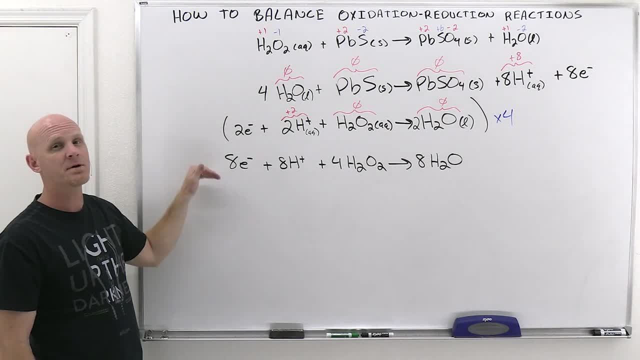 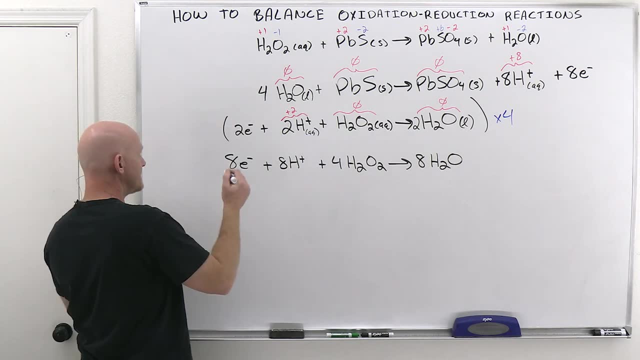 And now that the first half reaction and the second half reaction are balanced to the same number electrons, Now we can add them together. Normally, we've written both of these over again, So I'm going to write this top one over again, even though nothing has really changed. 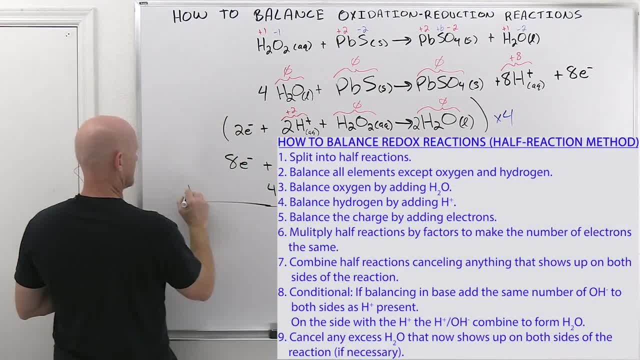 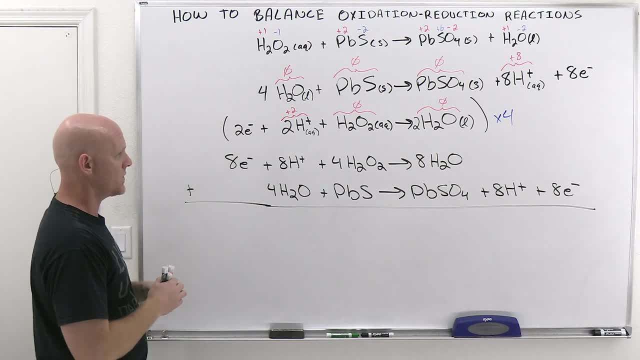 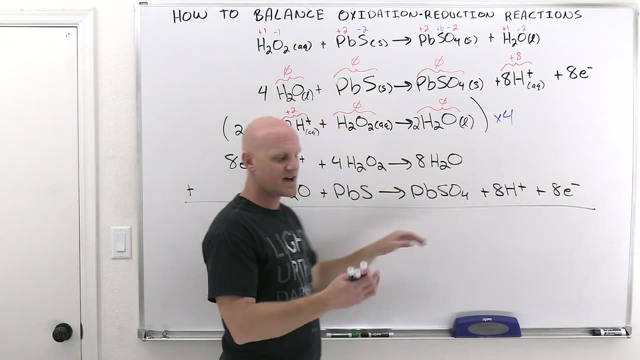 So that way we can add these two half reactions Together. Anything that shows up on both sides is going to cancel, but I'll worry about that in just a little bit. So we're going to put all the reactants together on one side of an arrow and all the products of both combined half reactions together on the other side of the arrow. 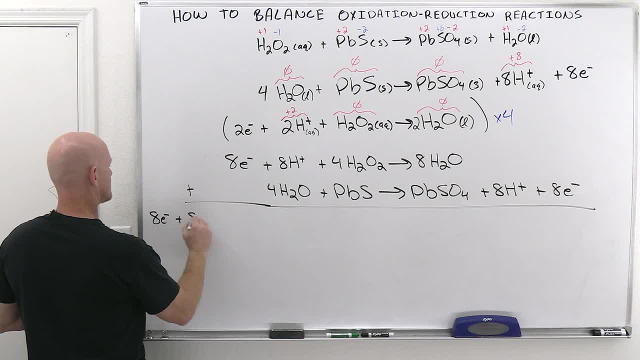 So in this case we're going to have eight electrons plus eight H plus. That doesn't look like eight H plus. There we go- Looks better- Plus four H2O2. and now the reaction to the second one as well. 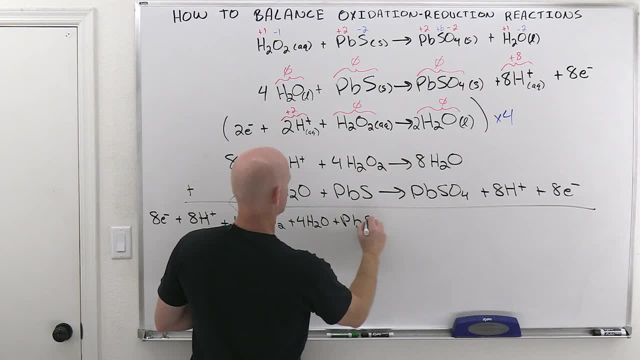 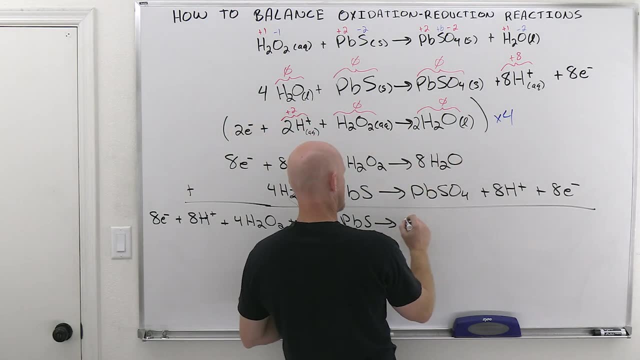 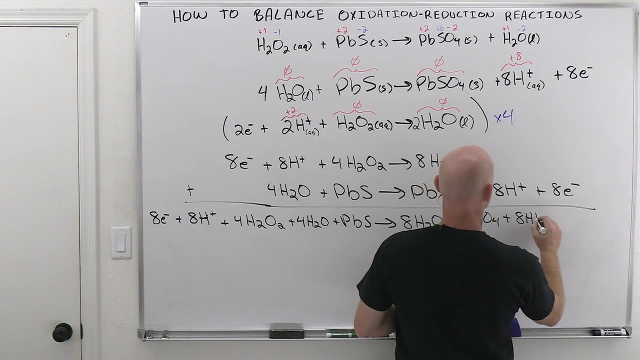 So plus four H2O plus PBS, and so all the reactants combined on the one side of the arrow and then all the products on the other side, And so eight H2O plus PBSO4 plus eight H plus plus eight electrons. Now, if you've done this correctly, 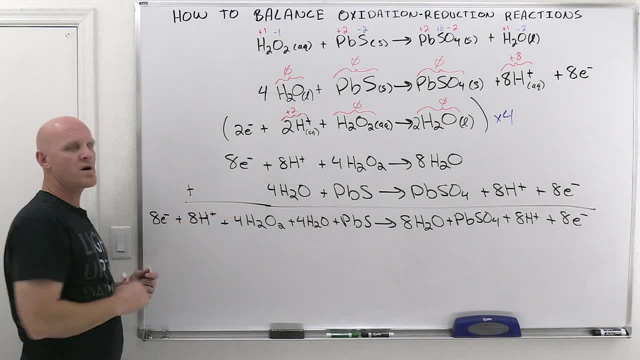 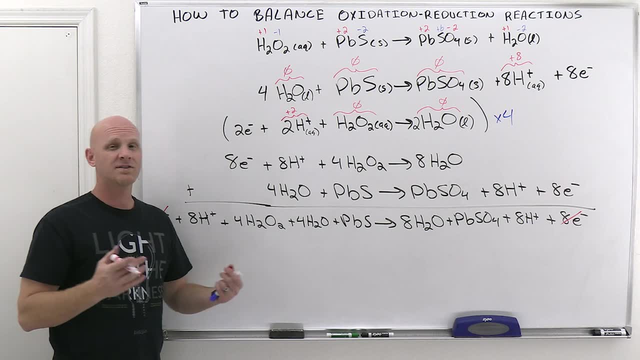 the electrons should cancel anything that shows up in the same quantity on both sides. Both sides is going to cancel. So these eight electrons are going to cancel out these eight electrons. but because H plus and H2O are often used to balance out auctions and hydrogen, 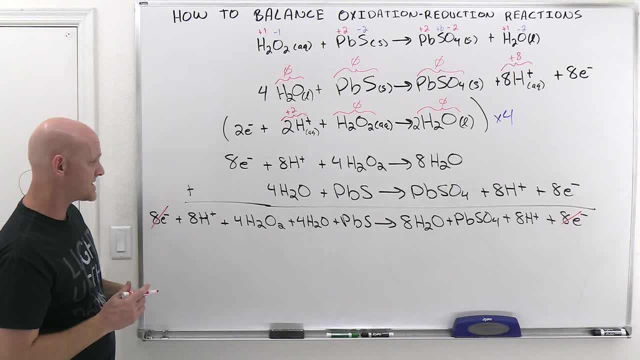 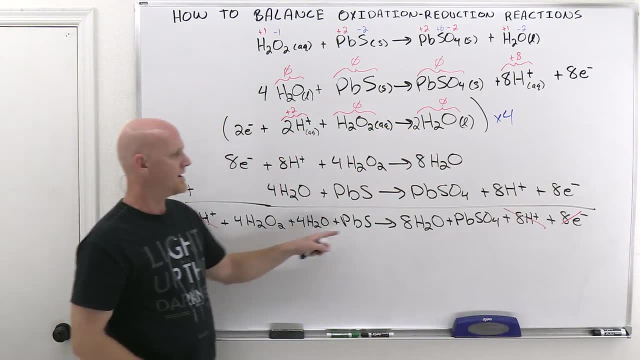 So commonly, you might have some of those showing up in both of these, on both sides of this as well. as we do notice These eight H plus are going to cancel out these eight H plus and we don't have an equal number of waters on both side. 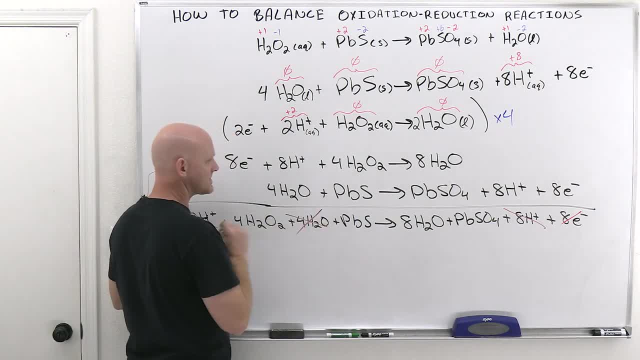 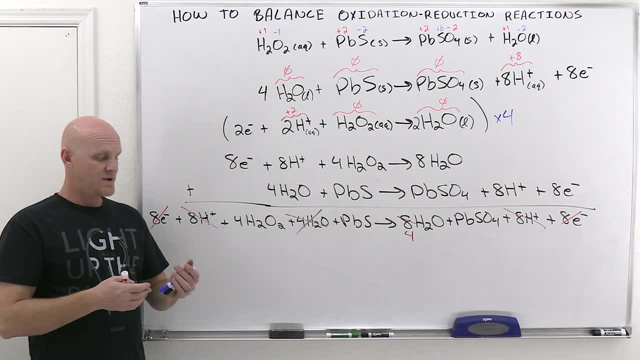 but we do have waters on both sides, and all four of these are going to cancel out four out of the eight of these, leaving us with four Left, and now we've cancelled out everything that we can cancel, And so what you've got left is your balanced reaction. 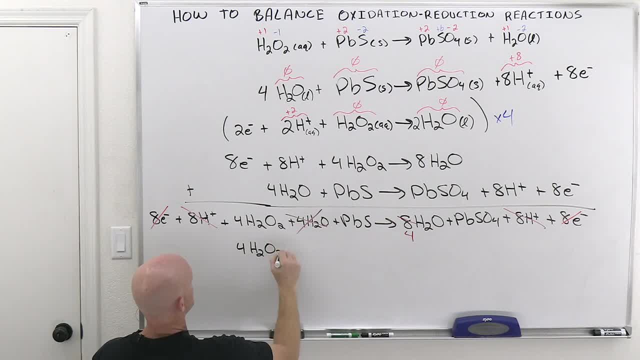 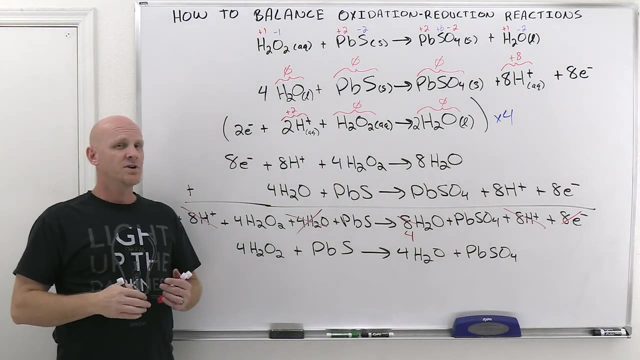 So in this case we've just got these four water- I'm sorry, these four peroxides right here, Hydrogen peroxides plus PBS, going to four waters plus PBSO4, and that's it. Cool. Now, by default, I said we balance reactions in acid. 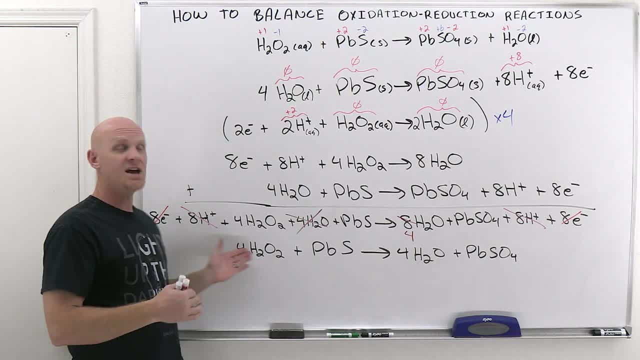 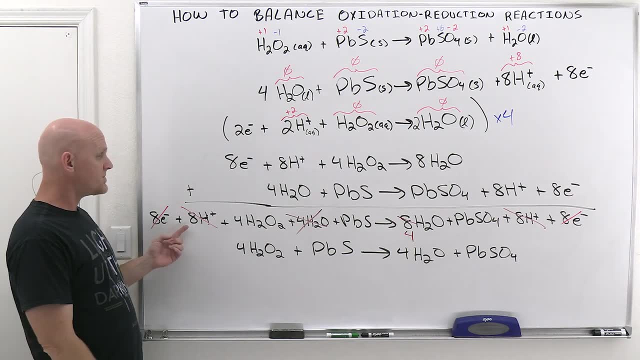 So, and usually the hallmark of a reaction that's been balanced in acid Is you see H plus in the reaction somewhere. The hallmark that it's been balanced in base is that you see OH minus in it somewhere. But in this example all the H plus is cancelled. 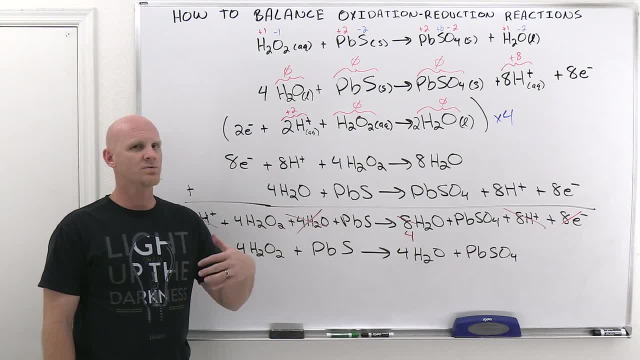 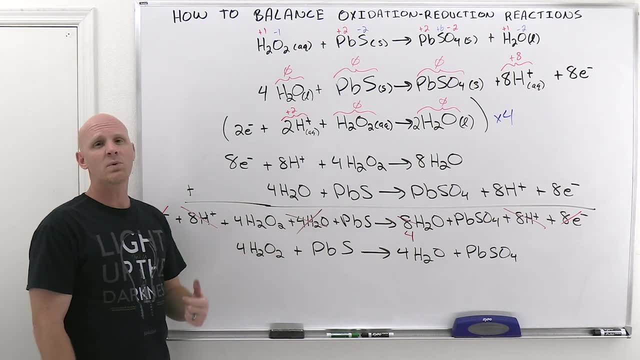 And so for this rare example, you actually couldn't tell the difference of whether it was balanced in acid or base, and because there's no H plus or OH minus in the overall balanced reaction, And so in this case they wouldn't have to tell you to balance an acid or base. 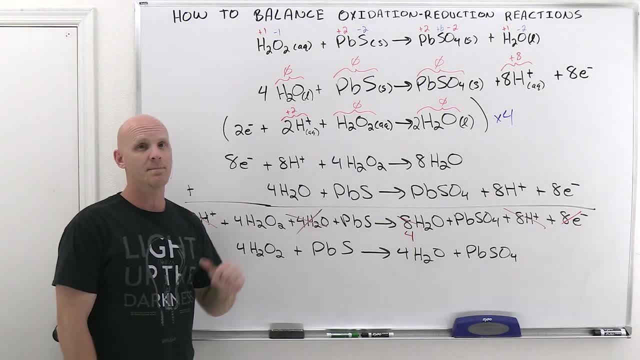 But most of the time when they give you a reaction, they have to specify: balance this reaction in acid or balance this reaction in base. if they don't tell you which, just proceed like normal, balance it an acid by default and you're probably going to find out that they didn't need to tell you. 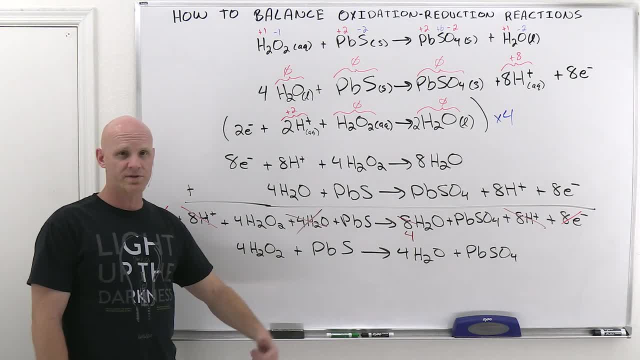 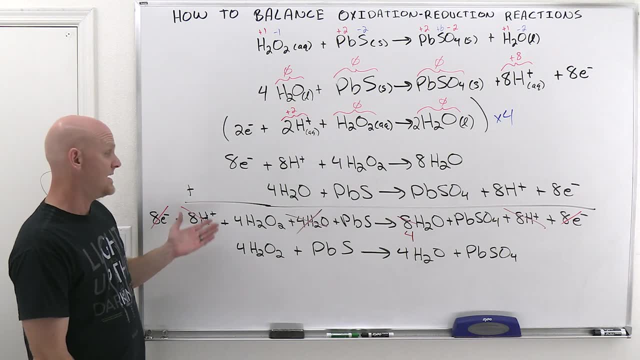 because it was an example like this where it would make no difference whether you balance an acid or base. it works out exactly the same because there's no H plus left over in the overall reaction. Cool. One other thing to note is you can check these at the end. 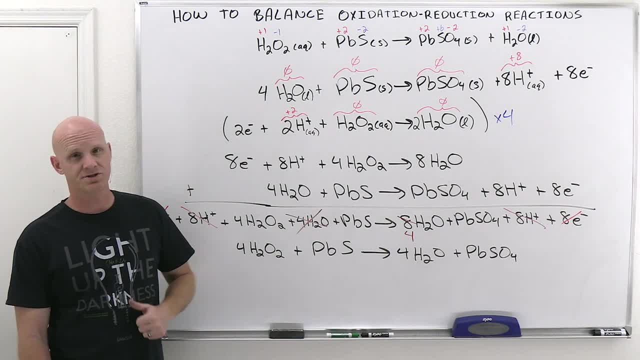 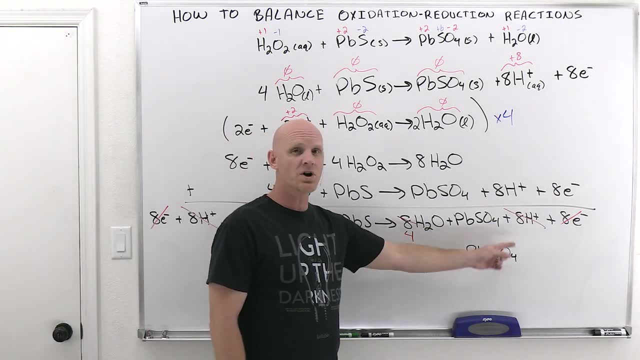 If you have properly balanced this, the overall charges should be balanced as well. Well, these are both neutral compounds, So the overall charge on the reactant side is zero. These are both neutral compounds, So the overall charge on the product side is also zero. 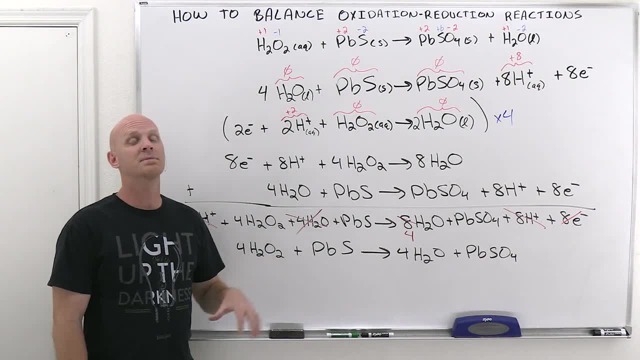 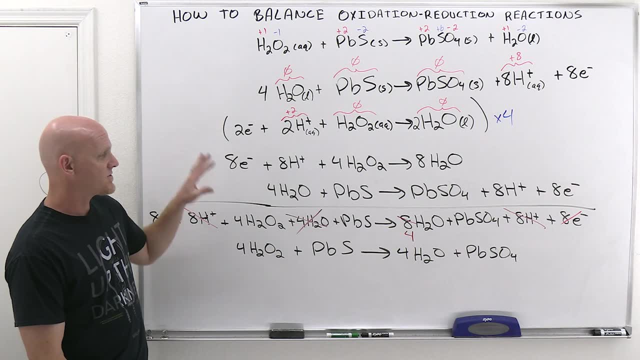 and the fact that those match doesn't for sure guarantee that it's right. But if they didn't match, then it would for sure guarantee that was wrong and you have to go back and figure out where your mistakes were All right. So that is our balanced reaction here. 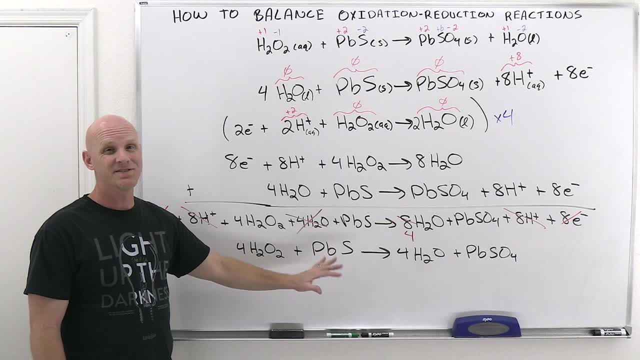 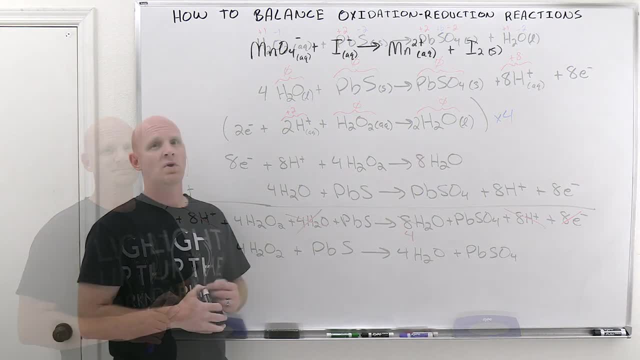 And again, that's the balance reaction and acid. That's the balance reaction and base in this example. In the next example we'll find out. it's going to look a little bit different whether we balance an acid or base, and we'll definitely do both. 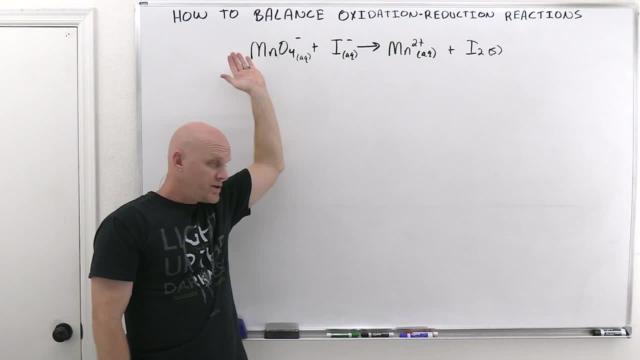 All right, Here's our second example here, And we could go through and assign oxidation states and figure out who's getting oxidized and who's getting reduced and which of the reactants is the oxidizing agent, which one's the reducing agent. 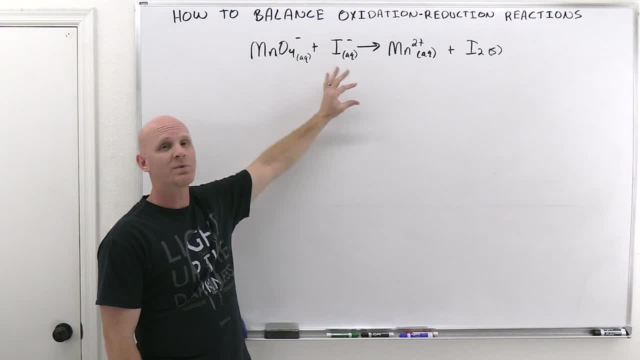 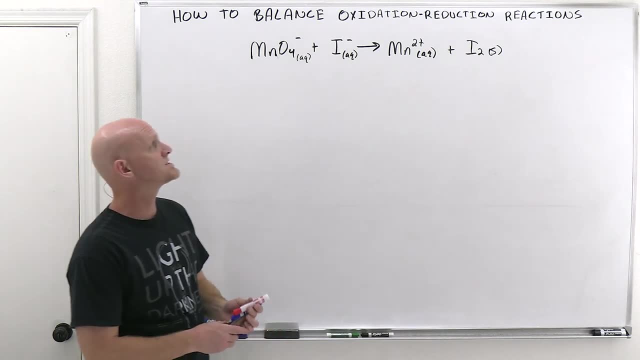 So, but we're going to do that at the end. I just want to make sure that you realize that to balance a redox reaction you actually don't have to assign those oxidation states first in using this half reaction method. So first thing I want to do is split this up into two half reactions. 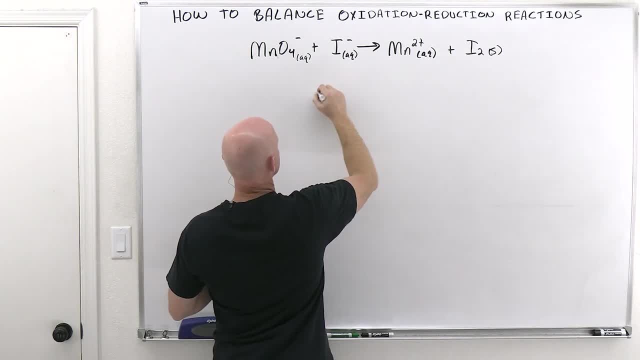 And in this case there's not a lot of options here. So you can pretty much see that we're going to have MnO4- going to Mn2 plus in one half and then I minus going to I2 in the other half. 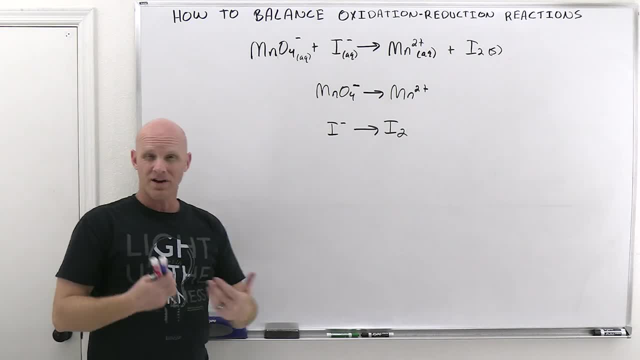 And so if you ever given a lot of more chemical species and stuff like that, you got to figure out which specific ones. So some words of the wise: if you see an element in its elemental form, it's in the zero oxidation state. 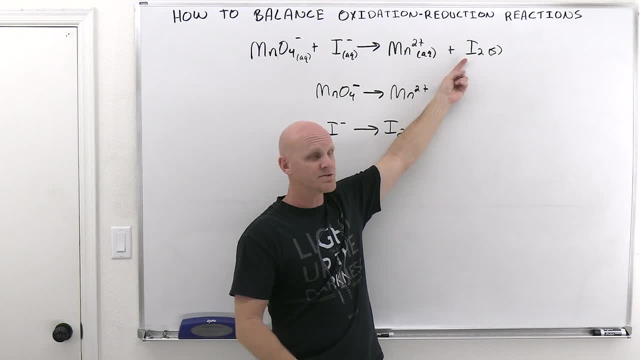 So in most elements don't have multiple allotropes, don't have like multiple elemental forms, And so if it's in the elemental form on one side, odds are it's not in the elemental form on the other side, And here it's zero, here it's not zero. 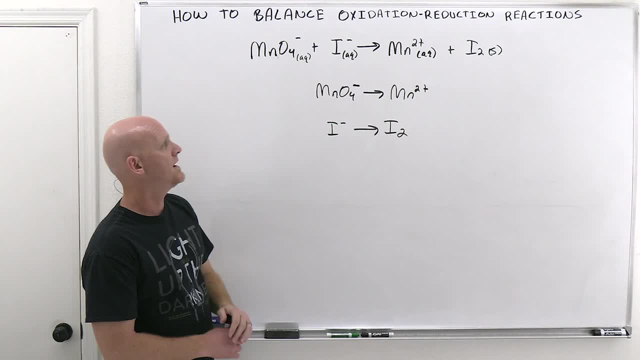 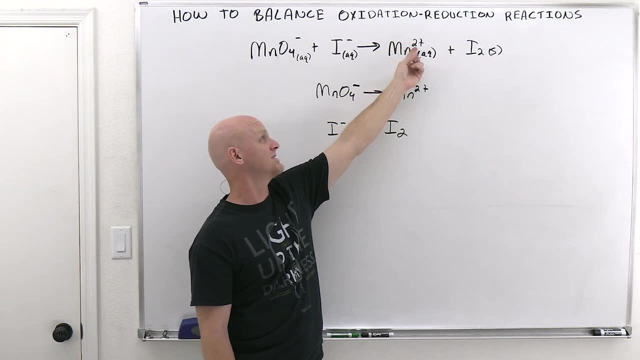 Yeah, that's changing. That should be in one half Of your, one of your half reactions. So the other one here. notice manganese as an ion and monatomic ion. It's just easy to see he's plus two And so you know. figuring what he is in this case is plus seven might be the way to go. 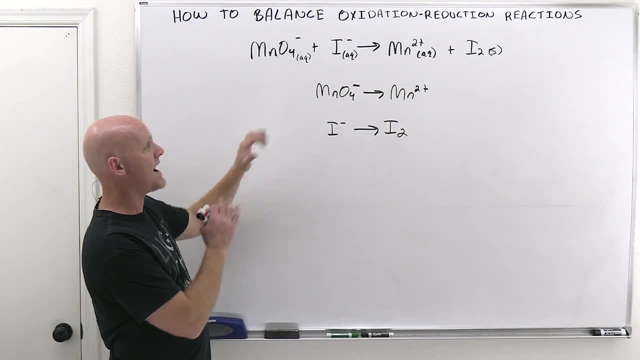 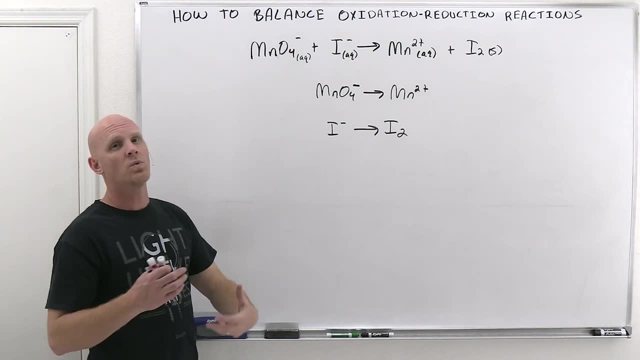 If you're trying to figure out who gets oxidized and who gets reduced, But again to do the half reactions here and solve this with the half reaction method. We don't have to assign oxidation states to start with at all, As long as you can identify what the half reactions are and split them up. 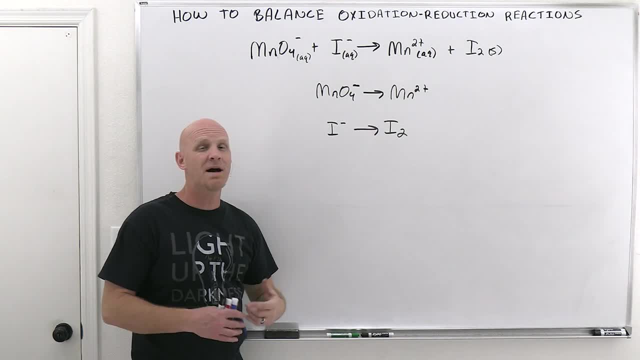 All right. So first thing I want to do, once we've split them up, Is balance all the elements except for oxygen and hydrogen. and the first one- The only other element besides oxygen, hydrogen- is manganese, and they're balanced. for the second one, It's iodine, and they're not balanced. 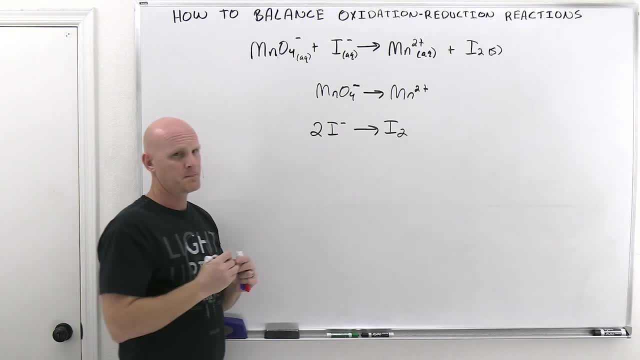 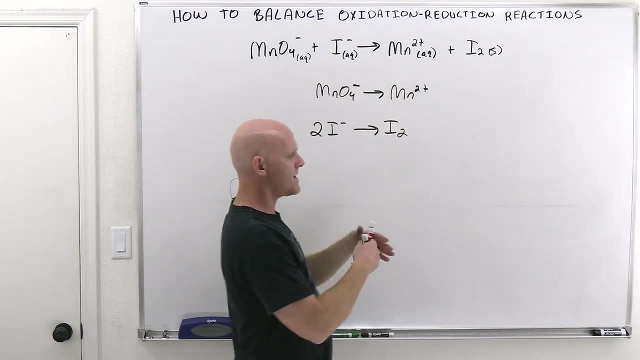 And so we're going to have to put a two right here. Next thing you want to do is then balance the oxygens by adding waters, and the first one. We've got four auctions on the reactant side, none on the product side, So we're going to need to add four waters. 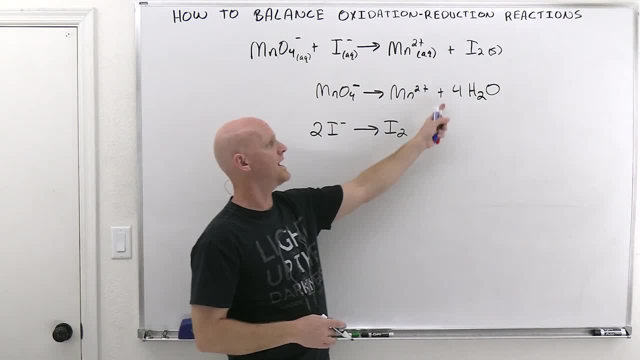 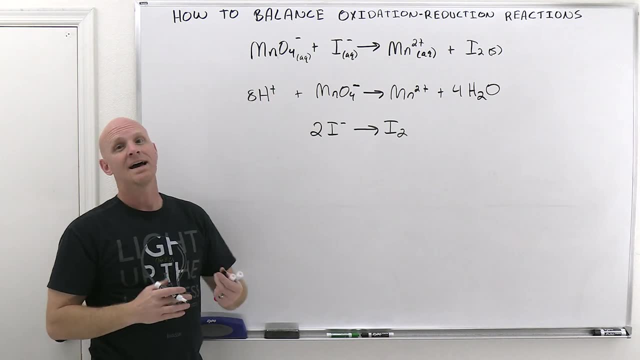 To make sure those auctions are balanced. but notice that throws off the hydrants. Now we got eight hydrants on the product side, none on the reactant side, So we'll have to add a H plus to balance those out. And now the auctions and hydrants for the first one are balanced and the second one doesn't involve auction or hydrants. 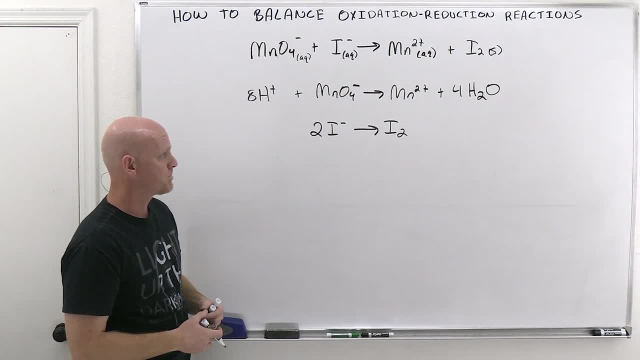 So we don't even have to incorporate waters or H plus or anything like that. Now that all the elements are balanced, We've got to balance out the electrons by balancing out the overall charge, And so here we can see that we've got eight H pluses. 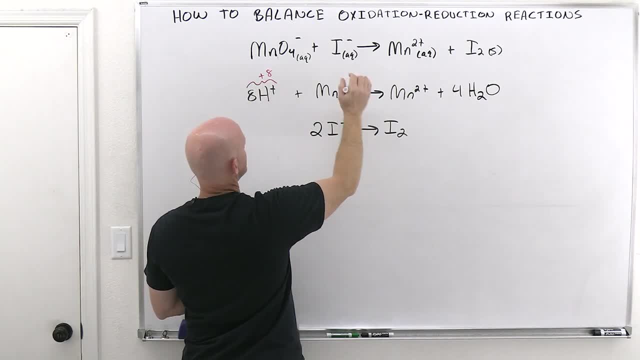 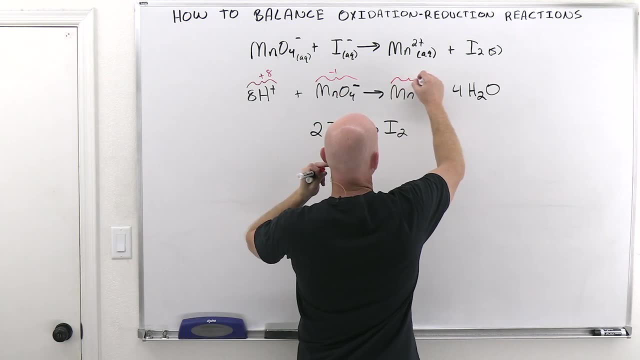 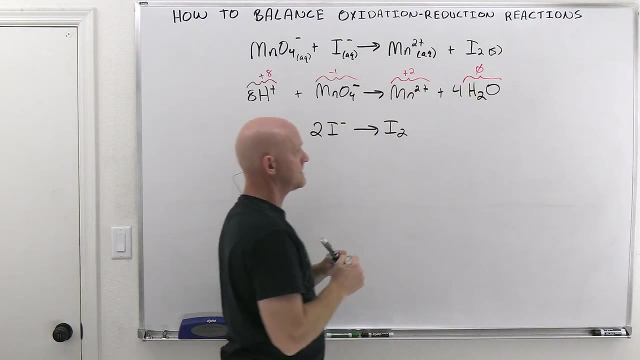 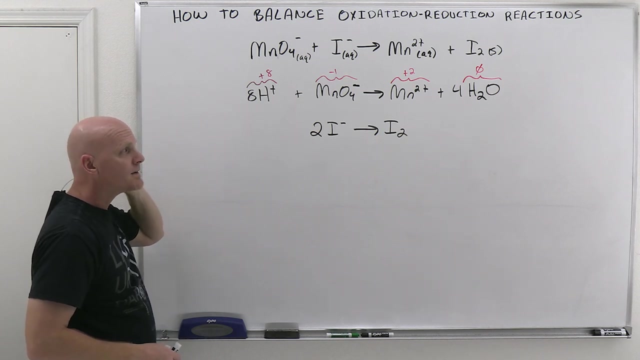 That's a total of plus eight. We've got one MnO4 minus an overall charge of minus one. Finally one manganese I on overall charge of plus two. And then water overall is neutral With no charge there. See if we can get that suit. 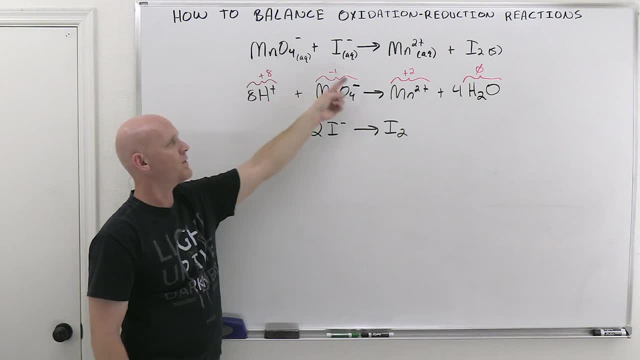 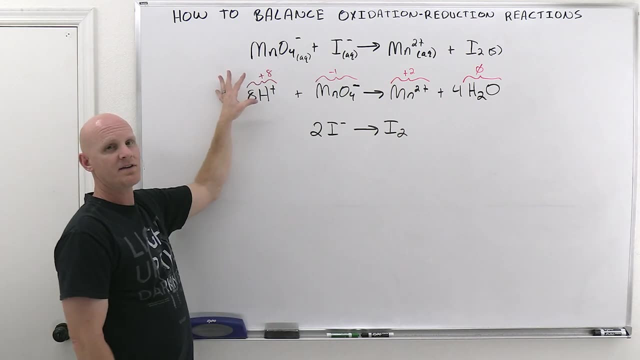 All right. so we can see that with eight pluses and one minus, the entire reactant side is plus seven, But the product side is a total of just plus two, And so this is the more positive side at plus seven, And we're going to have to have five charges- negative charges- to it to make it balance out to the same charge as the right hand side. 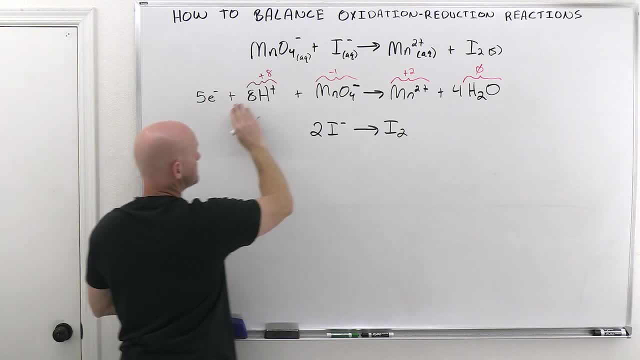 So, again, the goal here is- you have to realize, I'm not balancing it out to zero- just to have both sides have the same charge. And so, with it being plus seven, we need seven electrons. We only needed five to now, both sides being plus two. 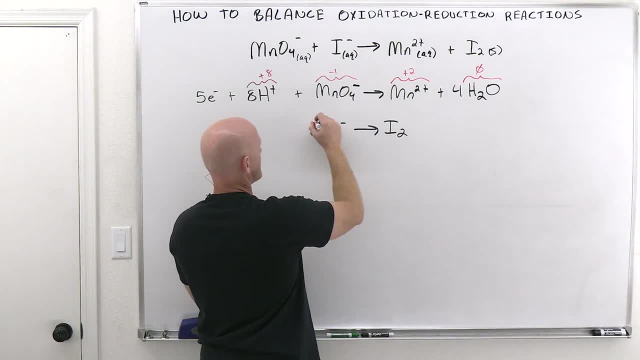 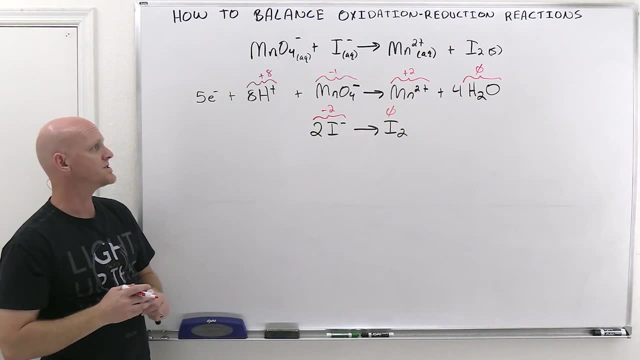 And the next one. here we've got two iodide ions for a total charge of minus two, And then iodine is an element in its elemental form. It has no overall charge, And so the more positive side is the right hand side, and we're going to need to add two electrons. 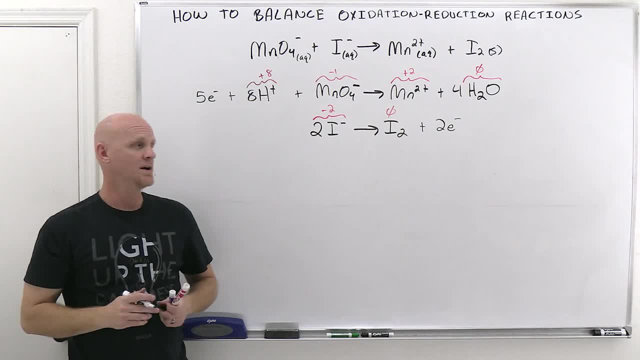 And now both sides have the same charge, in this case minus two. And so, once again, we're not adding electrons to make both sides have a zero charge, but to make both sides have the same charge, and you always add those electrons to whichever side is more positive. 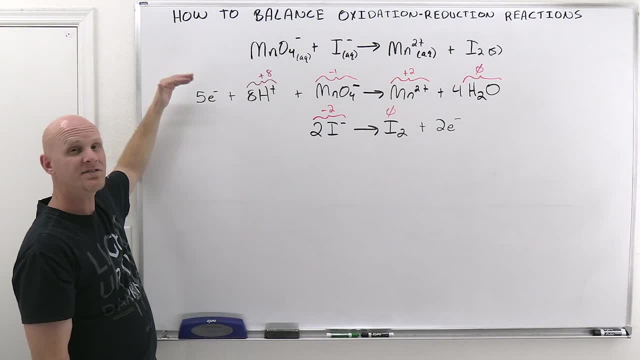 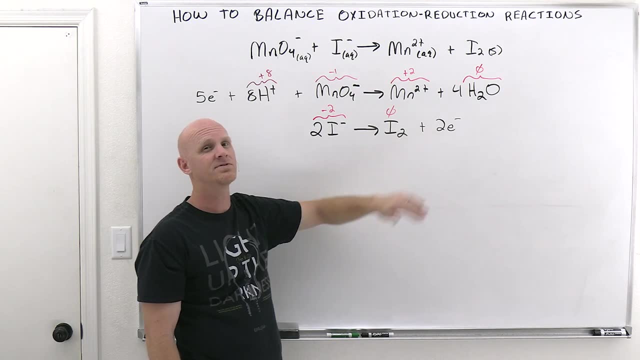 All right. so five electrons on the reactant side. These electrons are being gained. This is the reduction half of the reaction. So in here we've got two electrons on the product side. Those electrons are being lost. This is the oxidation half. 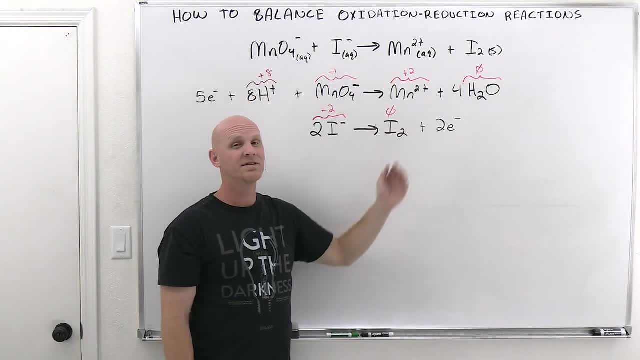 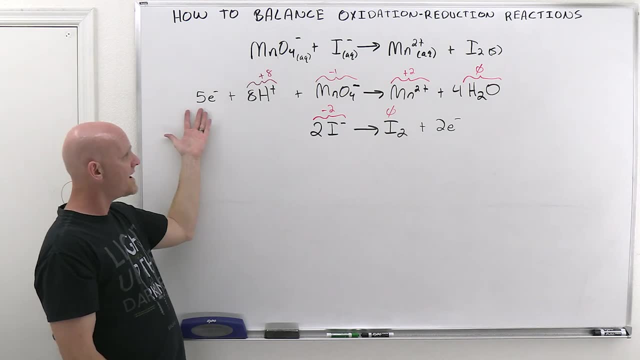 Of the reaction. but the electrons being gained here and the electrons being lost here are the same electrons, So they've got to be the same number. and you ask yourself, Okay, what is the least common multiple between five and two? and the least common multiple is 10.. 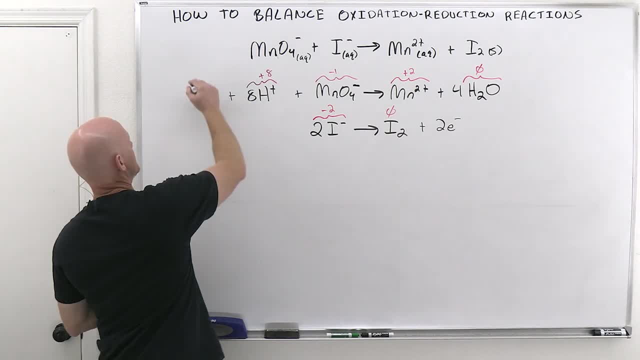 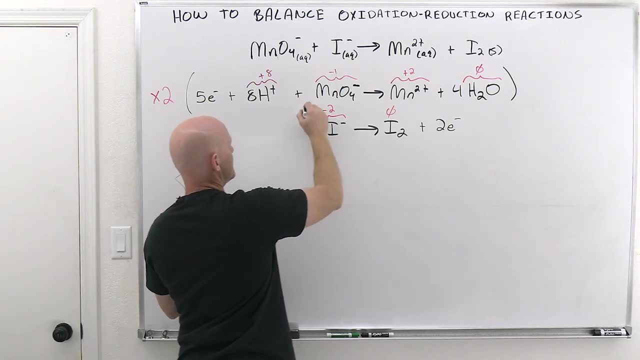 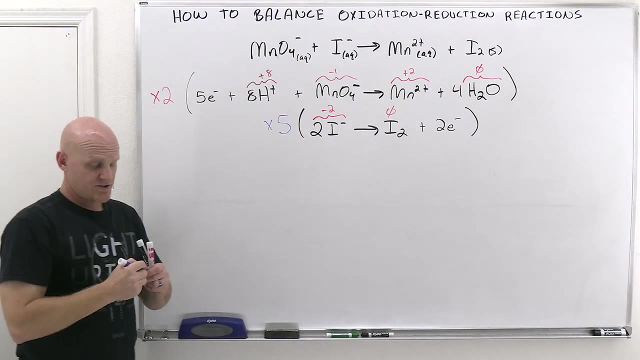 And how do you make both these balance out to being 10 electron processes? Well, for this one, you're going to multiply that by two, So, and for the second one, you're going to have to multiply that by five, And let's rewrite both these out. 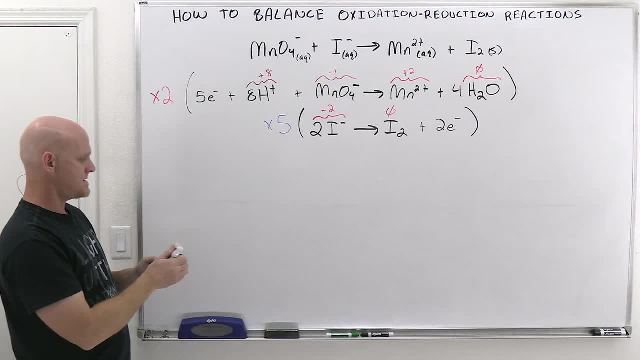 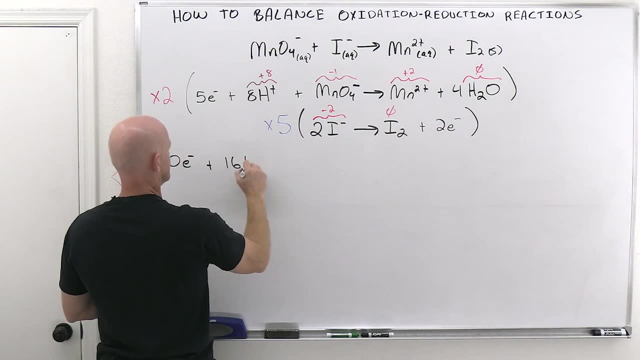 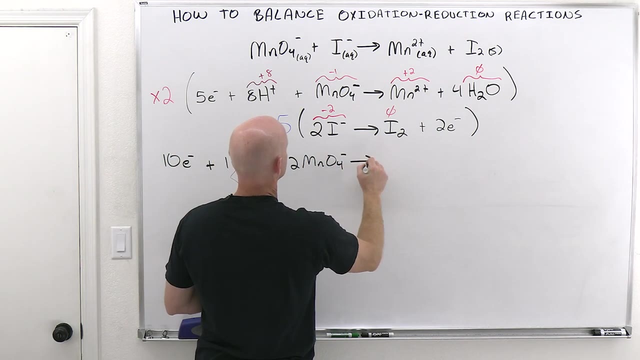 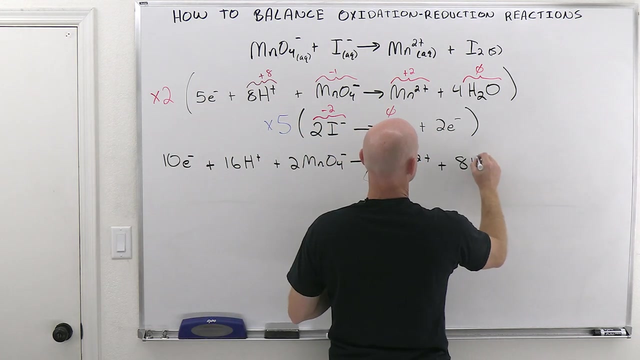 Once we multiply all coefficients by two and five respectively here, And so two times five is 10 electrons plus two times eight is 16h, plus two times One essentially, is two MnO4 minus goes to two Mn2 plus two times four is eight waters. 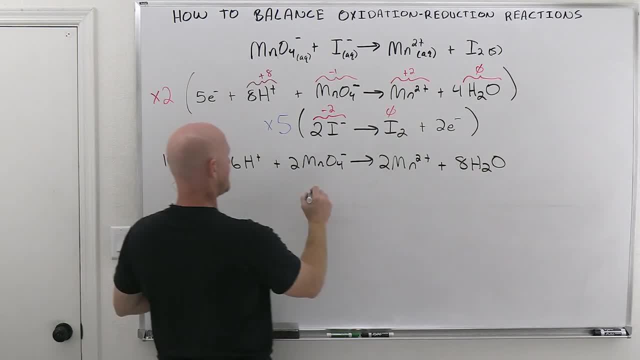 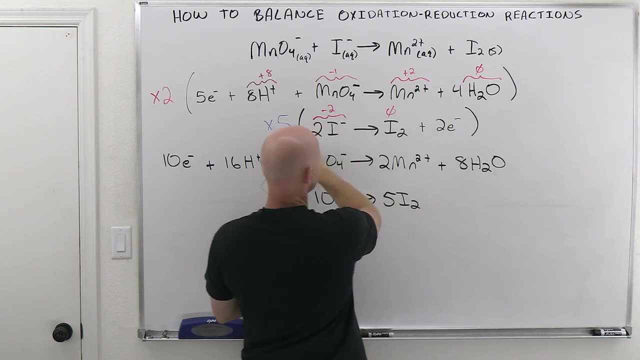 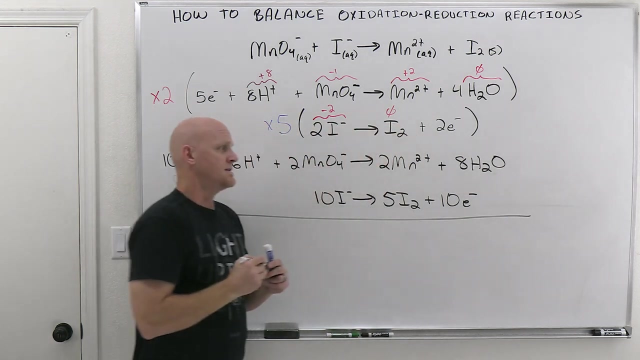 All right. And then this one times five. So five times two is 10.. I minus five, I two, and then five times two is 10 electrons, And this is what we ultimately want to add together. So in the last one I just kind of wrote it all out and then started cancelling things. 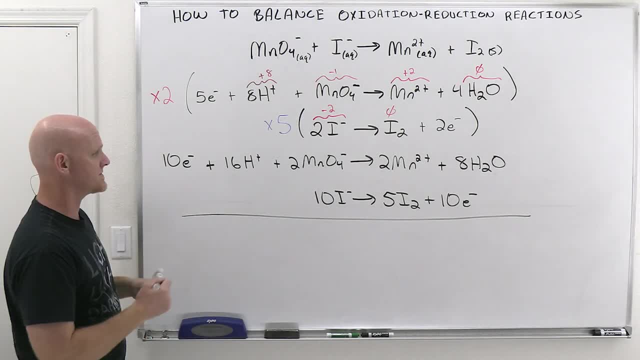 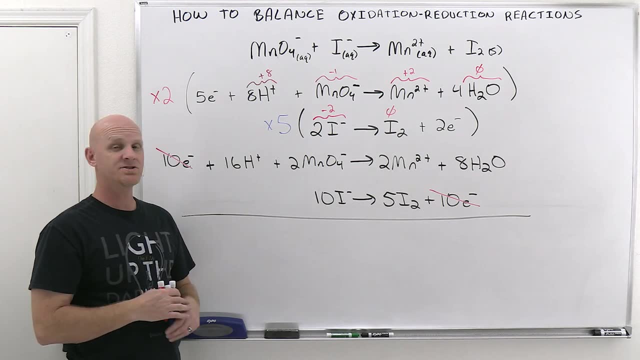 But you can kind of anticipate that some things are going to cancel. once you get used to these, We can definitely see that these electrons should cancel and again, and any properly balanced entire redox reaction. The electrons should not appear in it and they should definitely cancel. and from here, 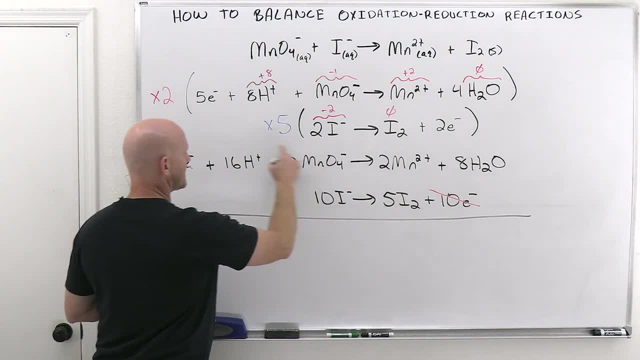 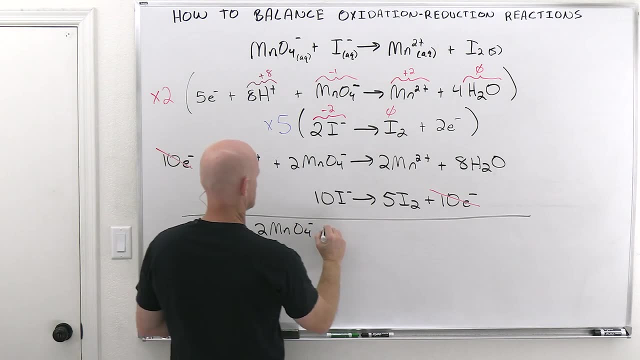 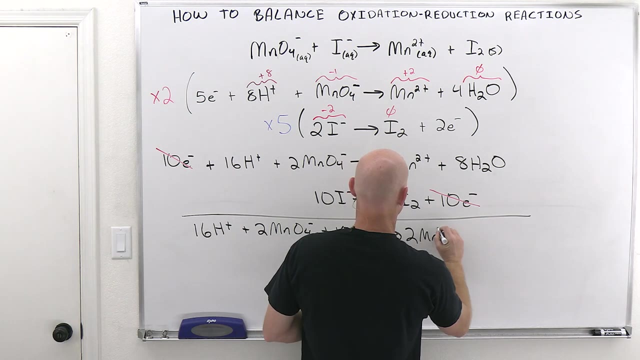 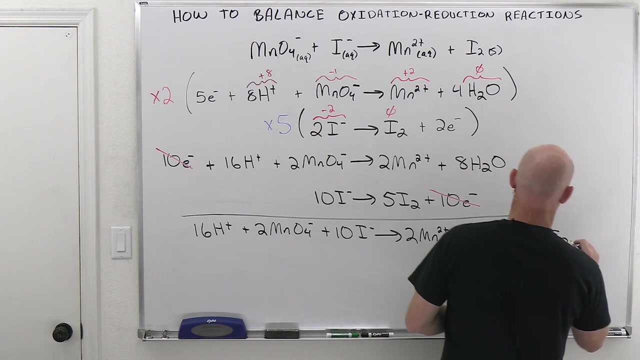 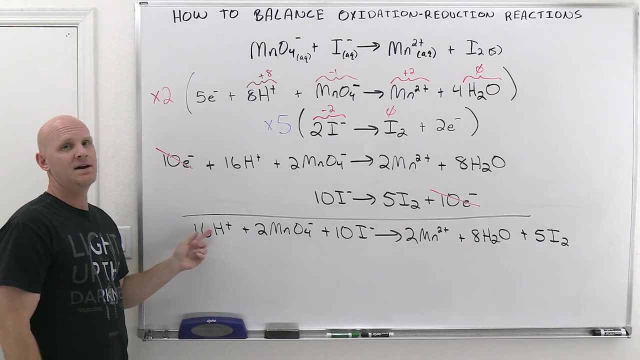 Nothing else is going to cancel. So let's just combine some terms here: All the reactants together on one side And then all the products on the other side. Cool, And this is the balanced reaction, specifically in by default acid. And again you can tell that a reaction has been balanced in acid because there's H plus either on the reactants or product side somewhere in the balance reaction. 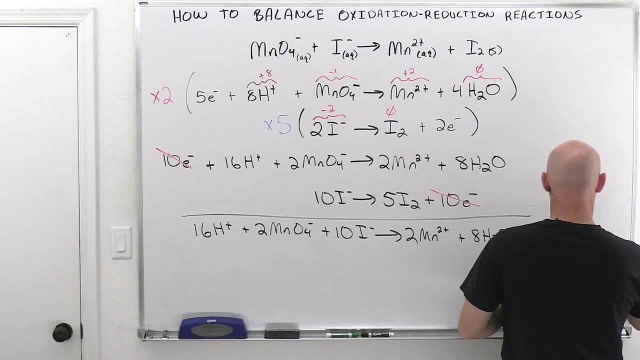 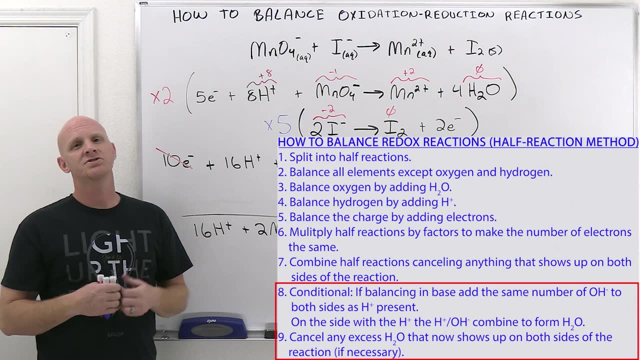 So this is the balance reaction in acid. If you're asked to balance this reaction in acid, you would be done So. however, if they'd asked you to balance it in base, you would have started out and worked this process all the way up till this step. exactly the same. 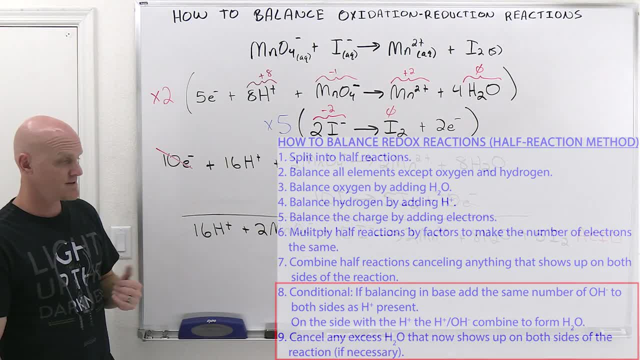 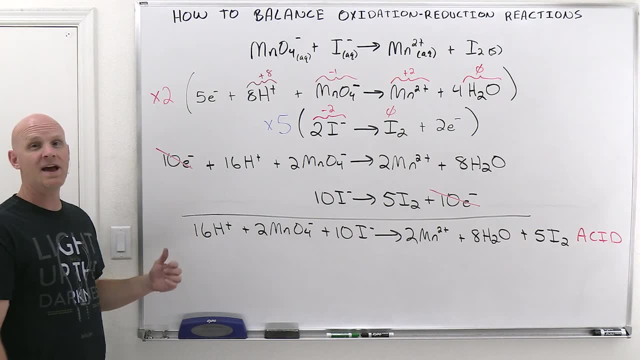 But you've got one extra step to do if you want to balance this in base. And you got to look at this balance reaction and say: well, what in this reaction would not exist in a basic solution to any appreciable extent? Well, that's H plus, because H plus would get neutralized in a basic solution. 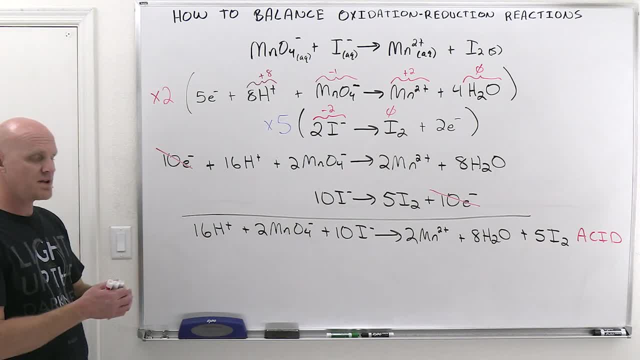 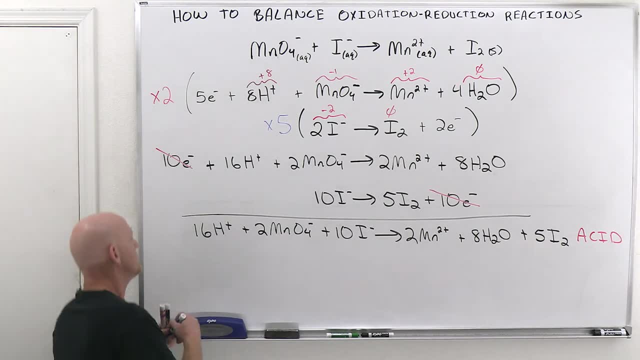 And that's exactly what you do. to balance this out is you neutralize all the H plus. Well, H plus gets neutralized by OH minus to form water, And so if you've got 16 of these H pluses, well, then you need to add 16 OH minuses. 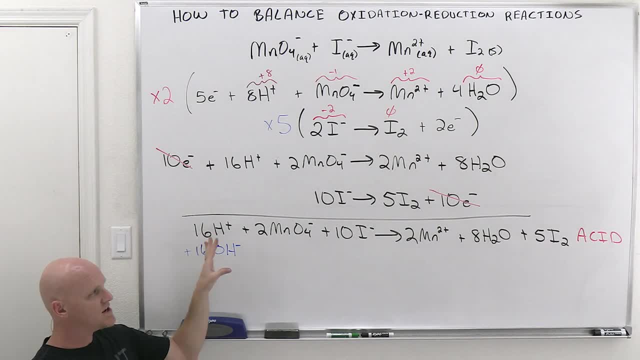 So, but we can't just do it on one side here, because a second ago this reaction was balanced in acid. It was balanced though, And so if we add 16 OH minuses only to the reactant side, it's no longer going to be balanced. 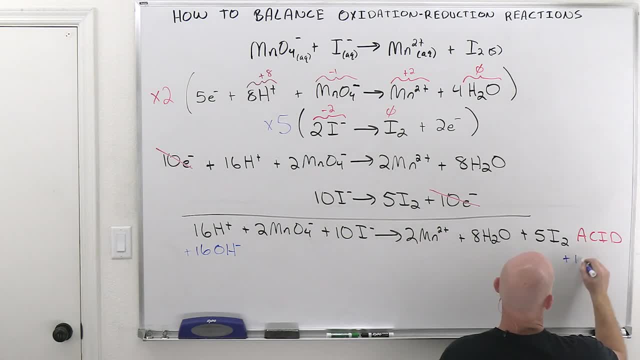 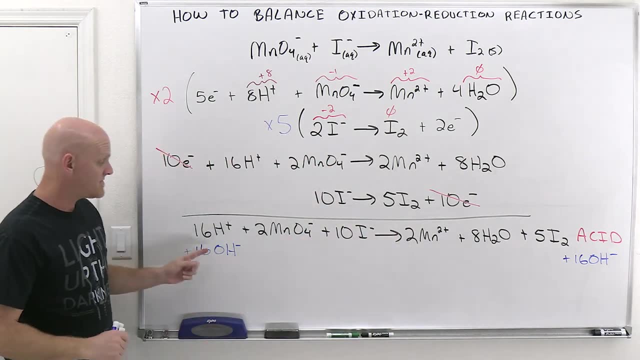 So we've also got to add 16 OH minuses to the product side. Now, on the product side it's not neutralizing anything, We're just adding it in. But on this side it's neutralizing H plus, And when H plus reacts with OH minus it forms water. 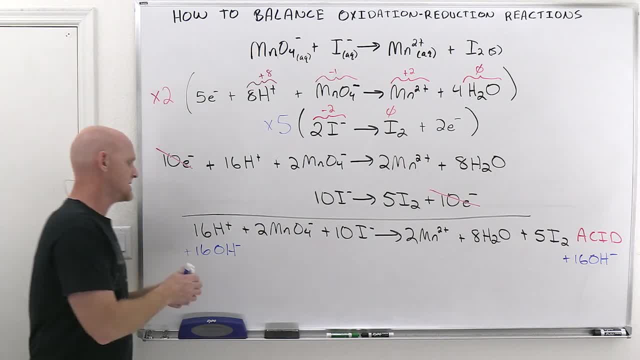 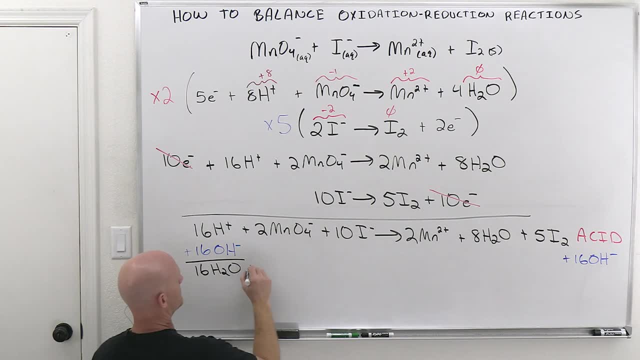 And so 16 H pluses reacting with 16 OH minuses Is going to form 16 waters And we'll add the rest in And we have these 16 OH minuses left on this side as well. Didn't neutralize anything. 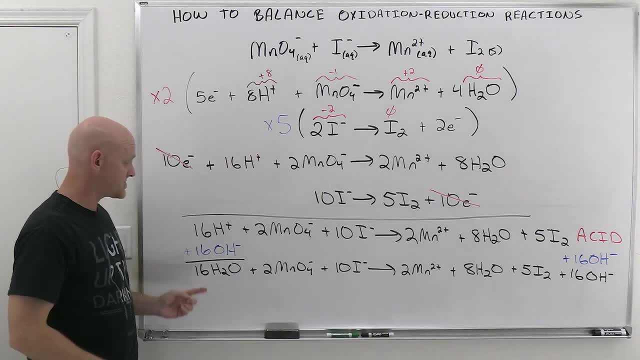 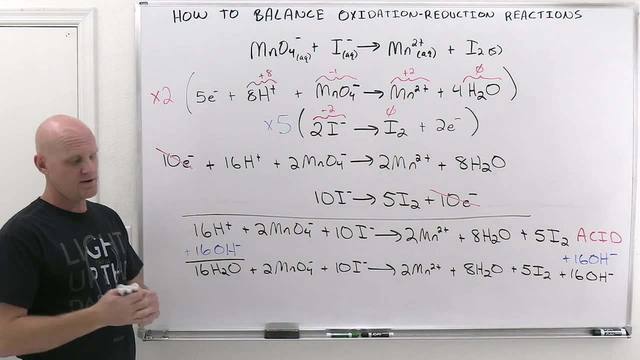 All right Now, because we just formed a bunch of waters over here And because water shows up so commonly- Because it's how we balance auctions- Now you should just check to see: did any of your waters cancel, since you formed a bunch of new ones? 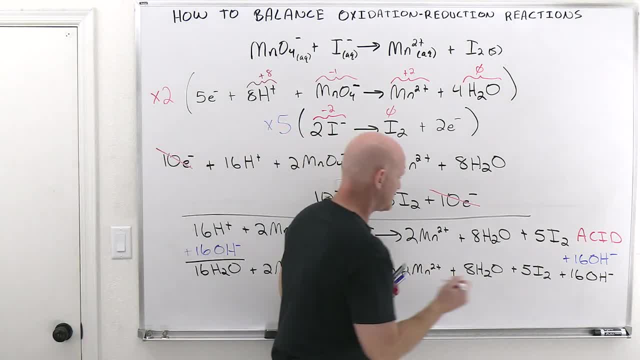 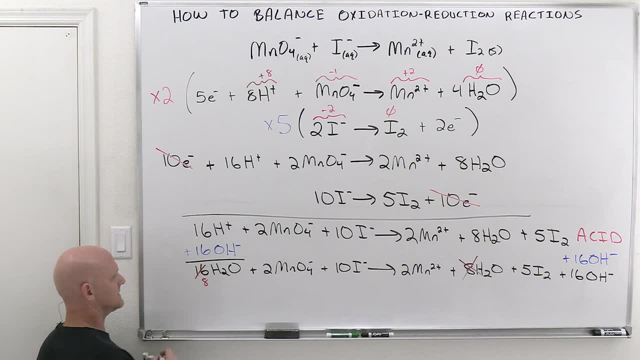 And it's totally true. We got 16 on this side, We got 8 on this side, And these 8 right here are going to cancel out 8 out of the 16 here, So that we only have 8 left. 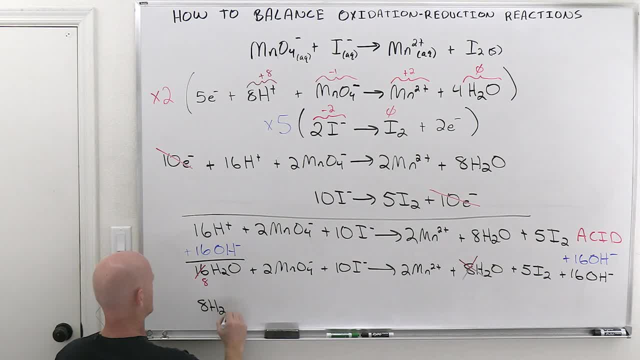 And we'll write this out one more time here. So 8 waters plus 2 MnO4 minus, plus 10 I minus Goes to 2 Mn2 plus no waters left on this side. So plus 5 I2 plus 16 OH minus. 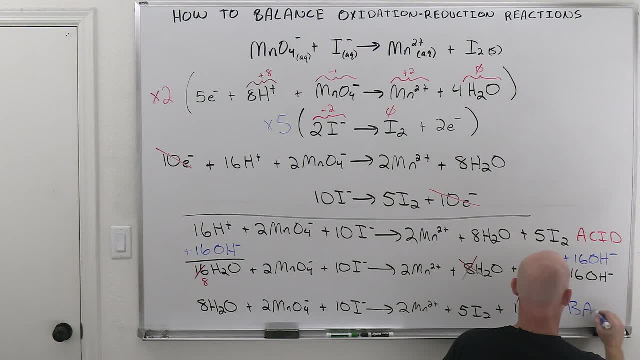 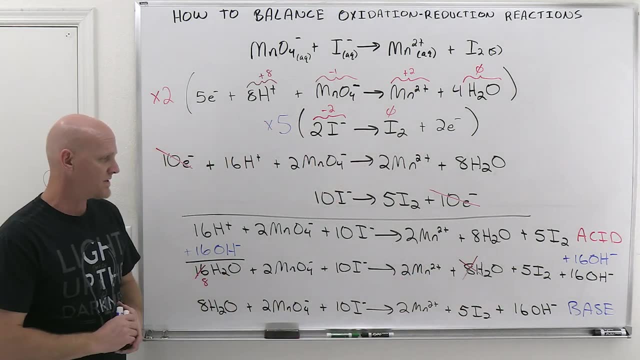 And this is the balanced reaction in base. And again, the evidence that it's been balanced in base is that there's hydroxide either on the reactant or product side somewhere in the balanced reaction. Now we said in the last example that you can check to see if you've done this correctly. 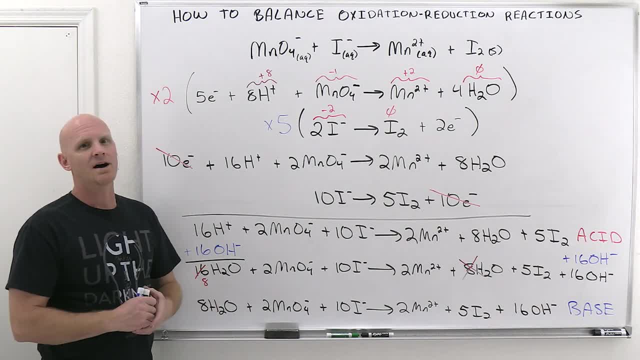 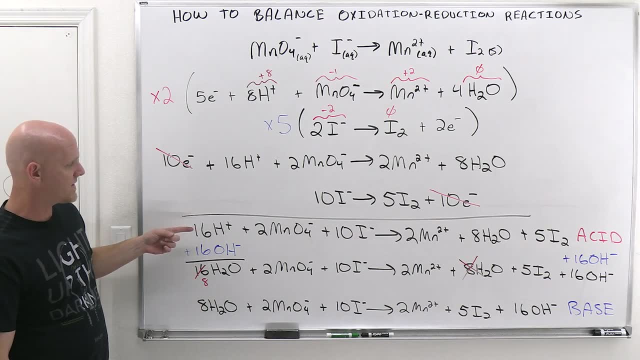 So at least you can check to see it very quickly If you've for sure done it incorrectly. Because in a properly balanced redox reaction, when you've all the electrons have been balanced itself the charge should be balanced. So here we've got in the acid form. 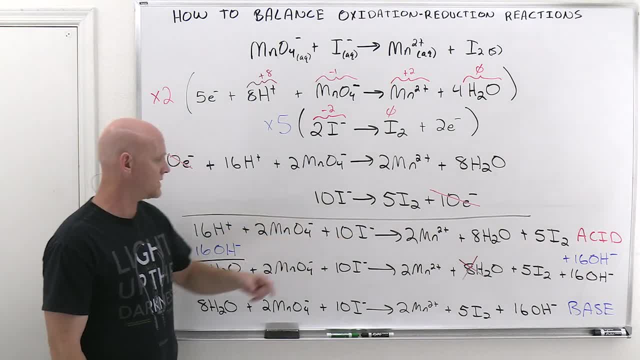 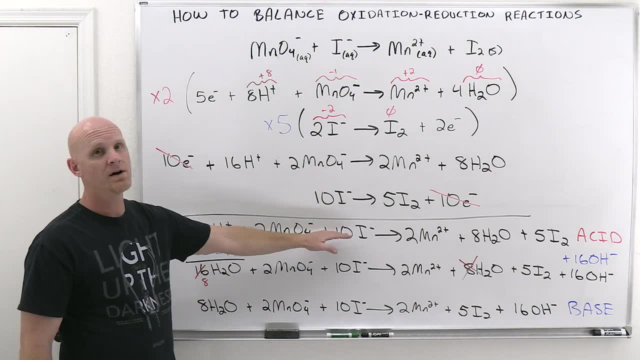 We had 16 plus ones, 2 minus ones, 10 more minus ones. So 16 positive, 2 negative. We're down to plus 14, 10 more negative. We're down to a total of plus 4 on the reactant side. 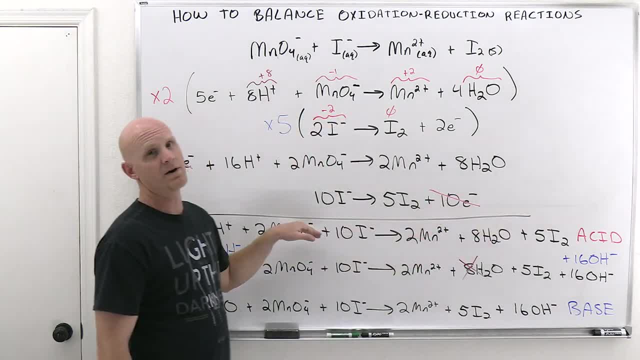 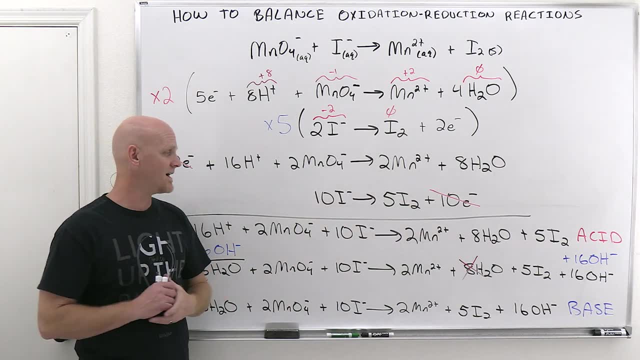 So 2 plus 2s is plus 4 and these are both neutral and it's plus 4.. And the fact that both sides have the same charge doesn't guarantee, again, that you've got it correct. But if they didn't match, it would guarantee that you didn't get it correct. 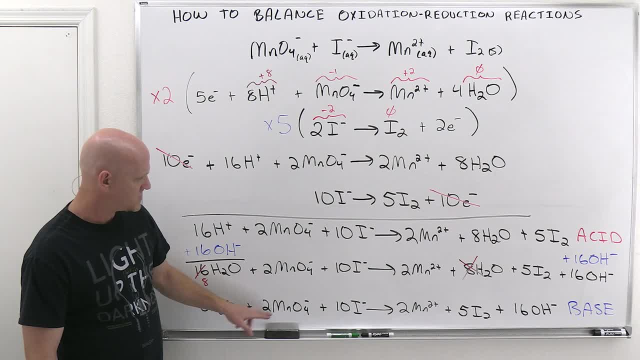 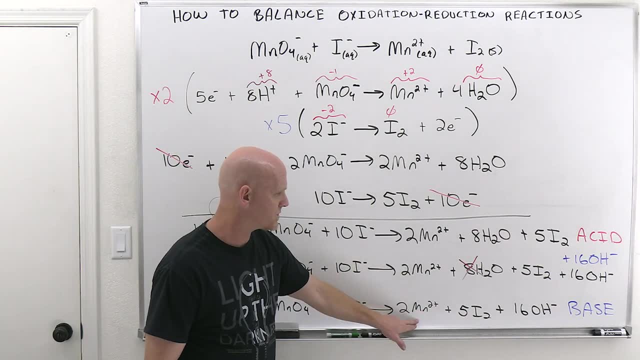 All right, same thing works out in base, In base neutral. but we got 2 minuses here, 10 more minuses here, for a total of minus 12 on the reactant side, And over here we've got 2 plus 2s, total plus 4 there. 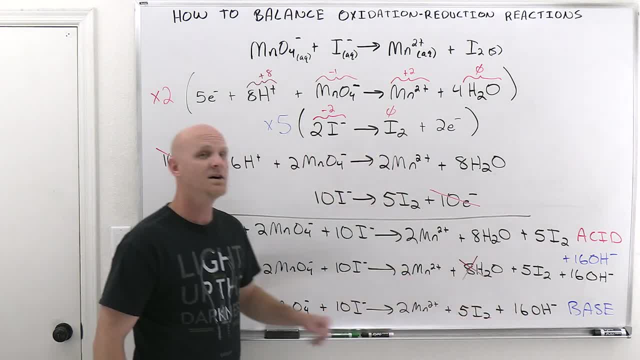 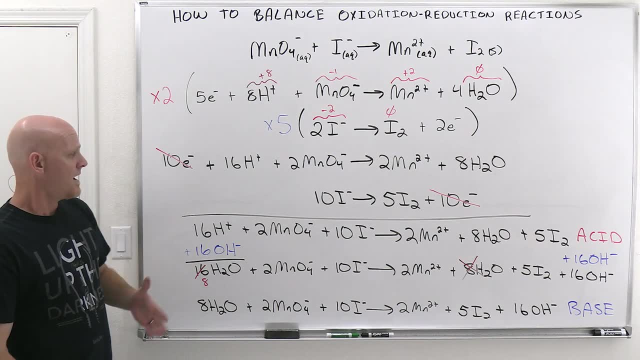 And then 16 minus ones over there, for a total of minus 12 on that side as well. And again, in any properly balanced redox reaction the charges should balance All right. one last thing here, And we'll just go back to the original. 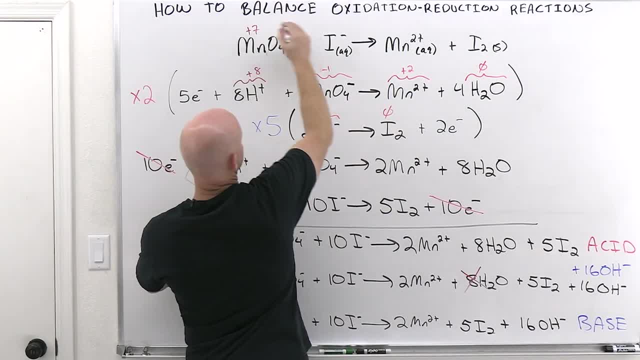 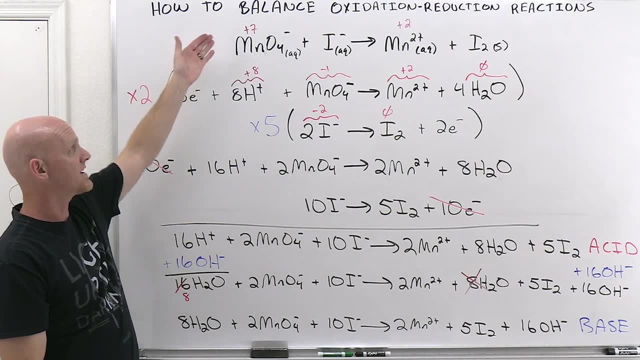 We said here that manganese is going from plus 7 and easy to identify as plus 2 here, And so manganese, there's oxidation state, is going down, It's getting reduced And so, because it's getting reduced, it is the oxidizing agent. 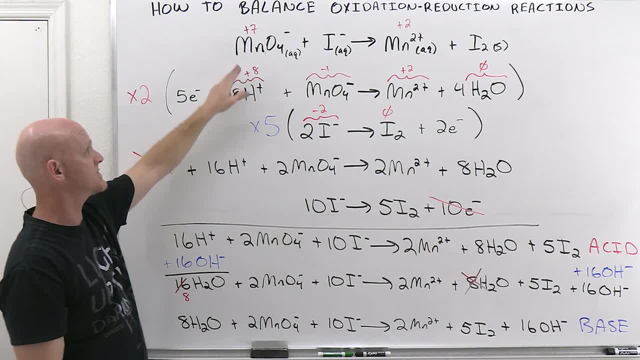 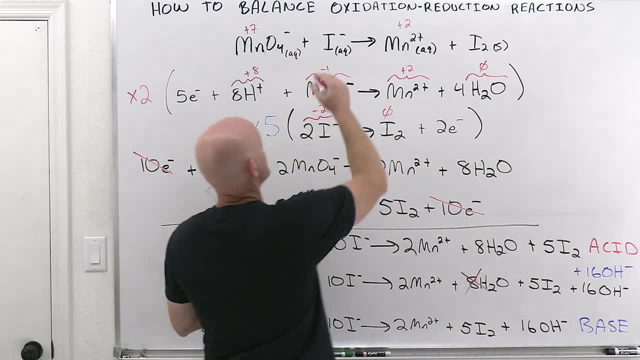 And we say it, we got to make sure again. we specifically say the entire species, So it's MnO4 minus that would be the oxidizing agent in this case. And over here we've got iodine in the minus 1 oxidation state going to iodine in the 0 oxidation state. 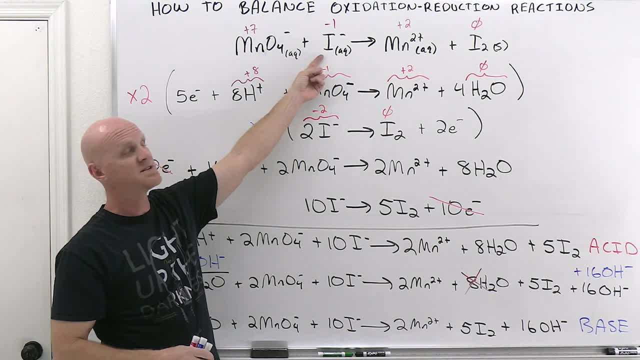 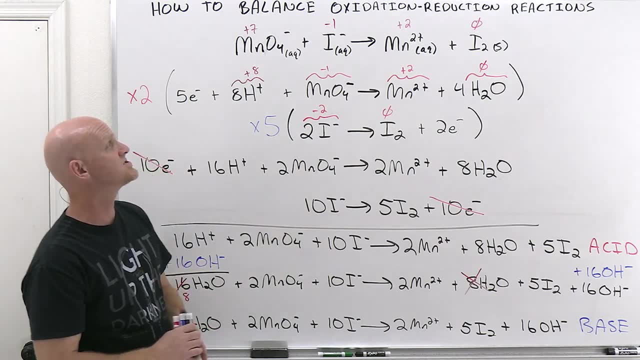 And so in this case that's getting oxidized. And because this is the species getting oxidized, it is the reducing agent. We typically not just say iodine, but I minus the iodide ion. in this case is the reducing agent as it's getting oxidized. 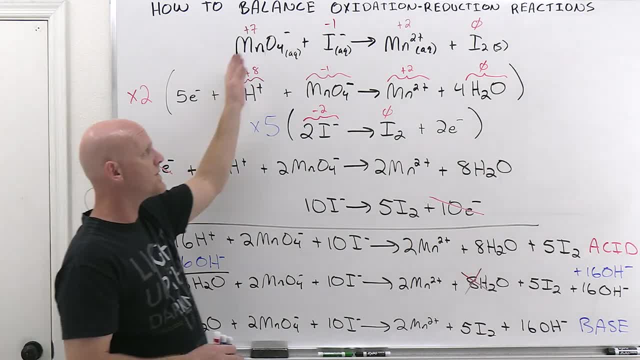 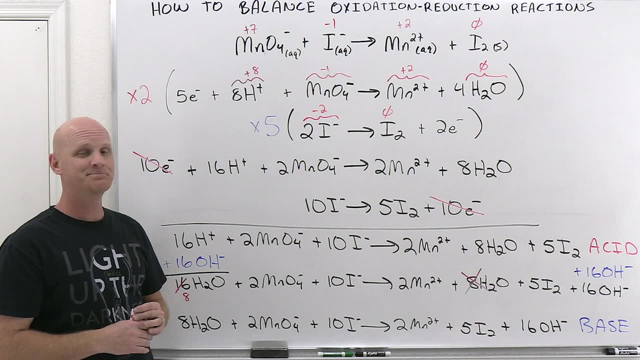 So just a reminder of how you identify those oxidizing, reducing agents. They're always on the reactant side And again it will seem a little bit backwards, So but hopefully what we discussed earlier kind of hits home at some point here, Just like it was with the oxidation number rules. 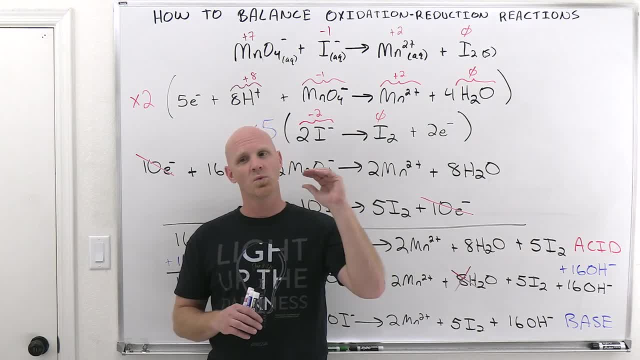 Best way to learn these rules: not simply look at the list and memorize them, But to work on them in the context of working out some examples. So keep those rules handy and just work your way through them. on some examples: best way to learn.